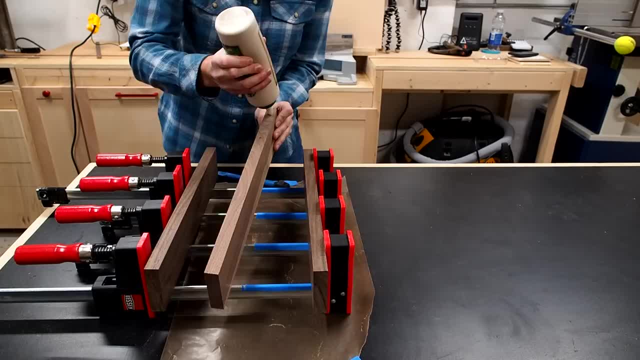 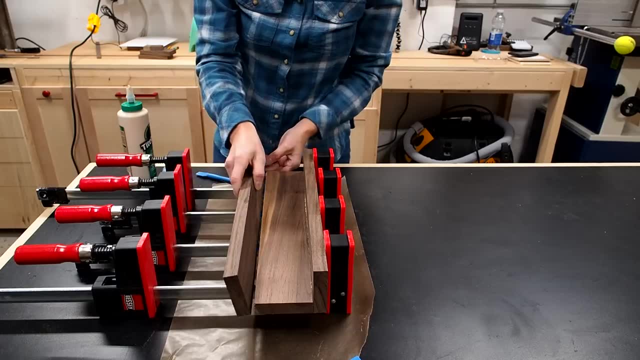 cut. I'll add some glue and assemble the pieces into a U shape, then clamp it and let it dry. And, by the way, you can find all the dimensions for all six projects in the written article over on my website. I'll leave a link to that down below. You'll notice the glue squeeze out. 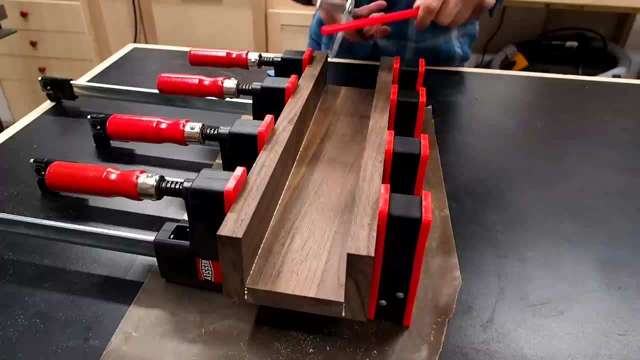 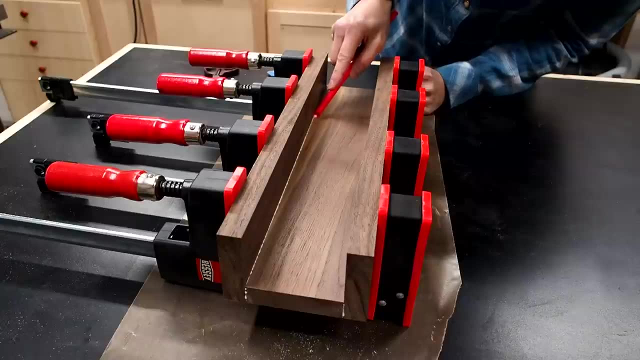 and that's exactly what you want to see. It means that you have enough glue on there. Cleaning it up can be annoying, though, so here's a simple little trick. I use a plastic straw that I cut on an angle and then kind of pinch the tip. 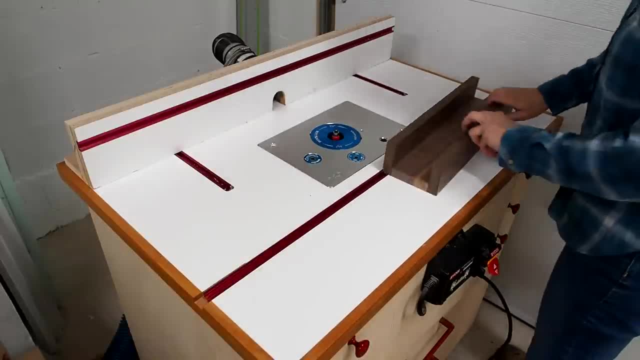 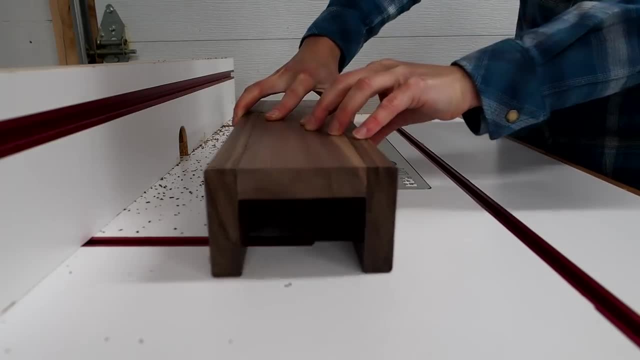 and run it along the inside crease Once dry. I'm going to round over all the edges to make it more comfortable to handle and it'll just look better too. I'm using my router table, but you can use a handheld router with a round over bit just as well. 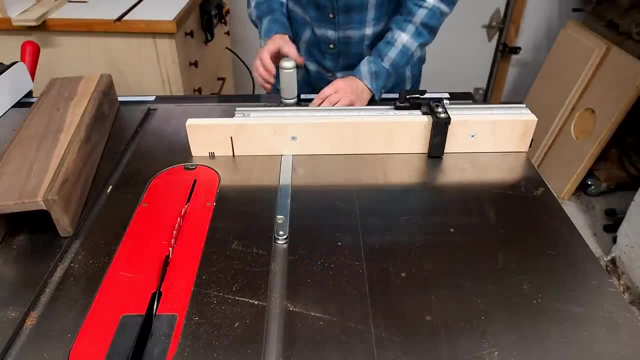 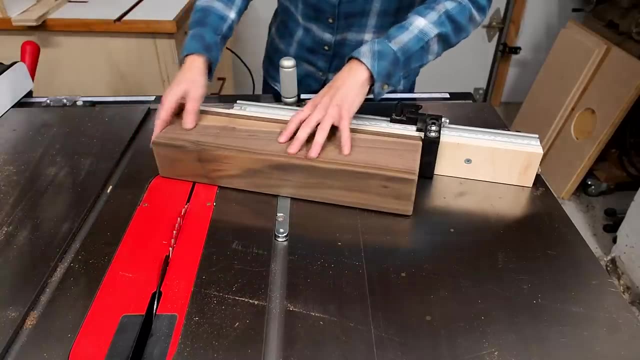 Next, I want to cut a slot to guide the bread knife as it slices the bread. Instead of making it perpendicular, I want it at a slight angle, so I'll rotate my miter gauge to say 15 degrees. I'm kind of nervous at this point. 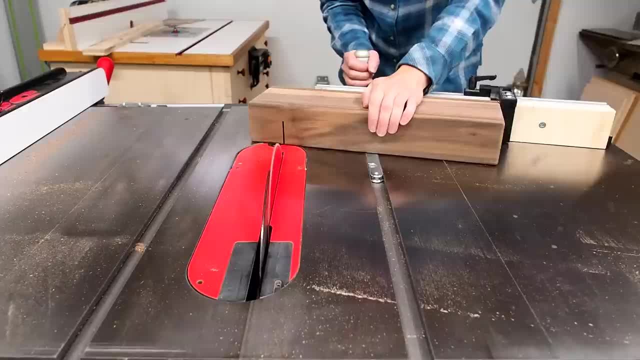 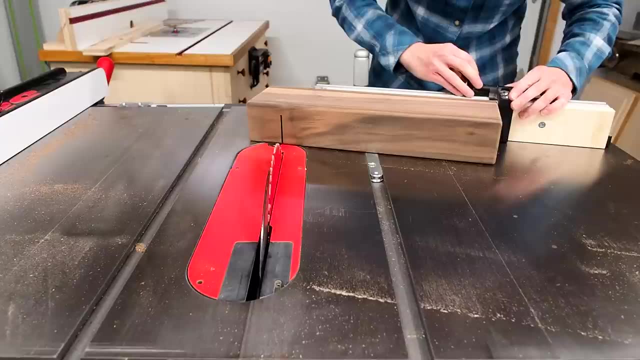 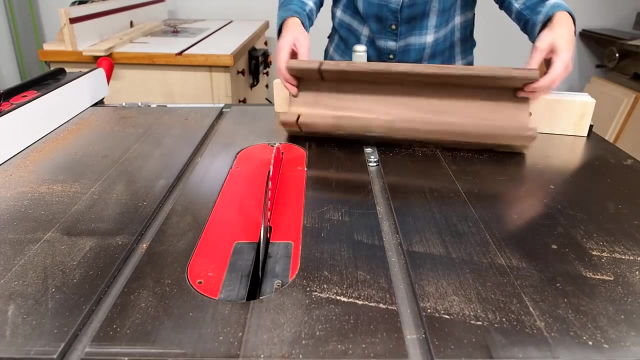 that I'm going to ruin my piece. so I took several passes raising the blade progressively until it skimmed the bottom, just barely cutting into it. I can then nudge it over a tiny bit and make another cut to widen the slot. I'll save you the boredom of sanding. 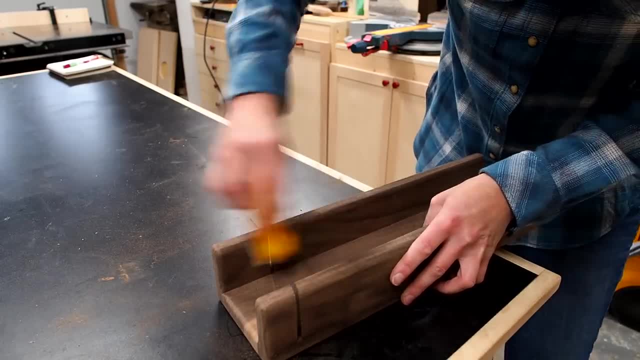 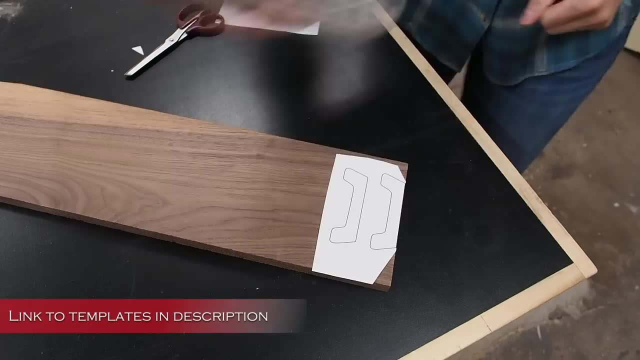 but just remember to sand folks. okay, I want to add some feet to this slicer, so I designed and printed these simple templates. I'll have these templates available on my website. if you want to print them out, I'll use some light spray adhesive to secure them to a piece of walnut. 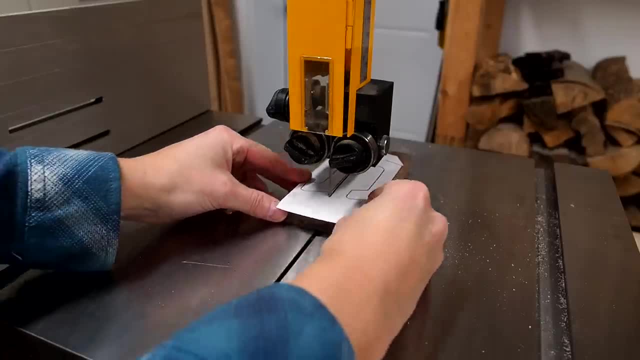 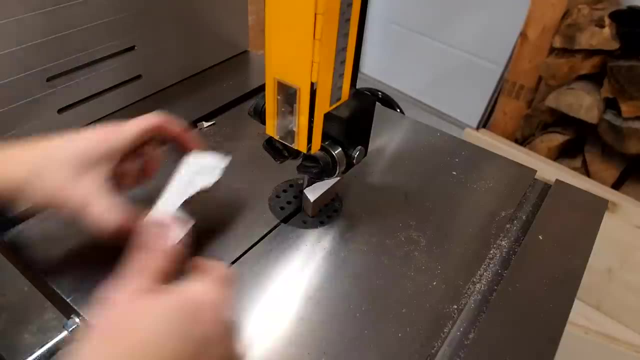 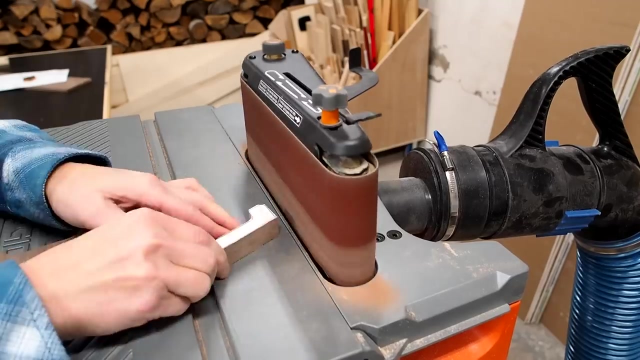 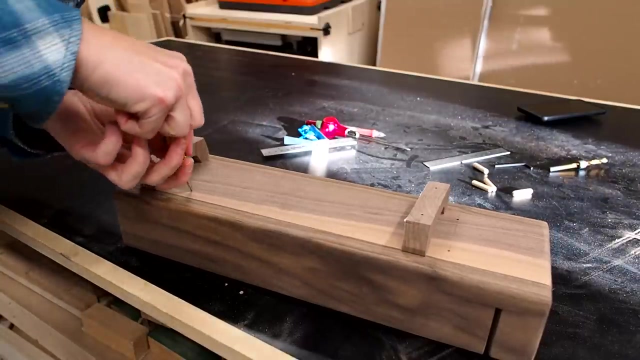 so I can then take them over to the bandsaw to cut them out. After cutting out a rough shape, I can refine it on the benchtop. All that's left is to attach the feet with a couple dowels. In hindsight, I think I could have just screwed them on from underneath. 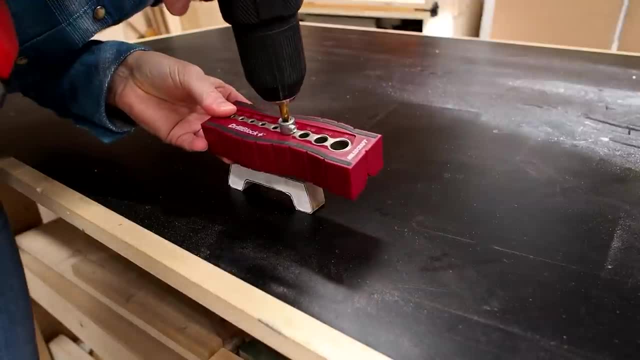 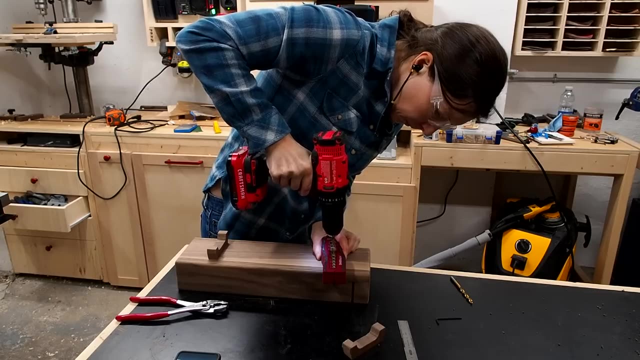 but of course I decided to make things complicated. I laid out my dowel placement and used a center punch to create a reference for the drill bit. I'll then use this drill block. that'll help keep my bit straight and make sure I don't drill too. 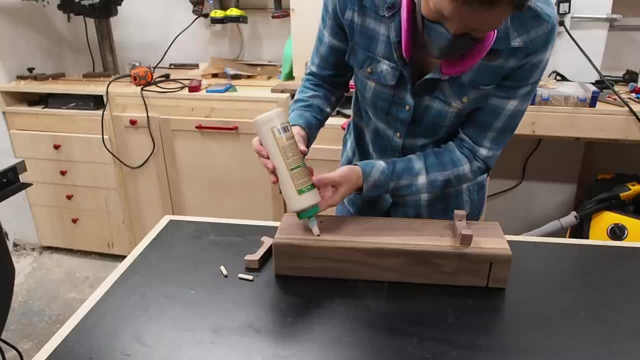 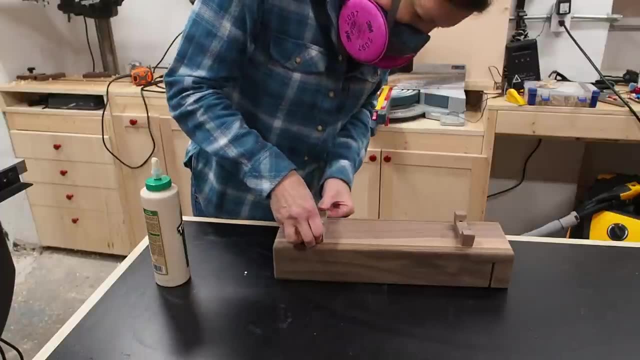 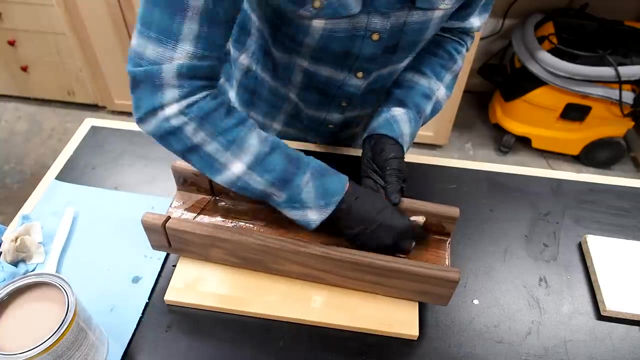 deep. Now I can simply add some glue and clamp until dry. Now all that's left is to apply a finish. I'll first wipe off all the dust using a tack cloth and apply two coats of Osmo Pollux oil. 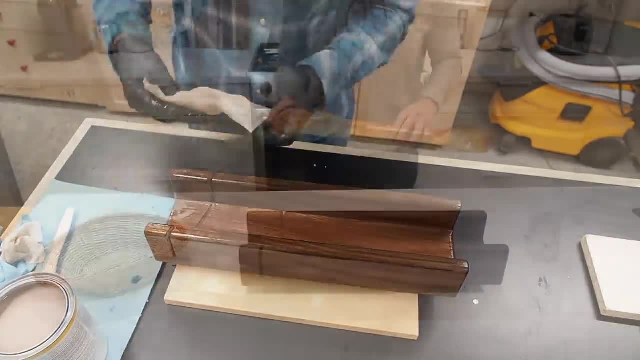 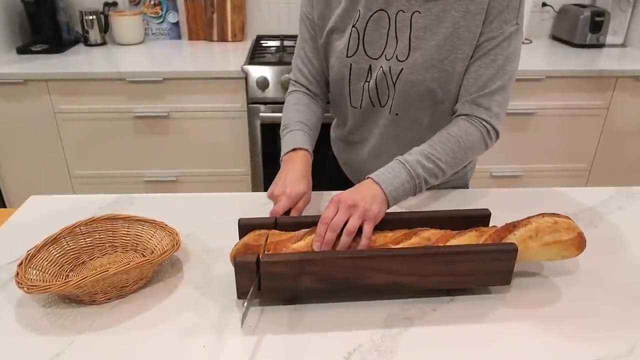 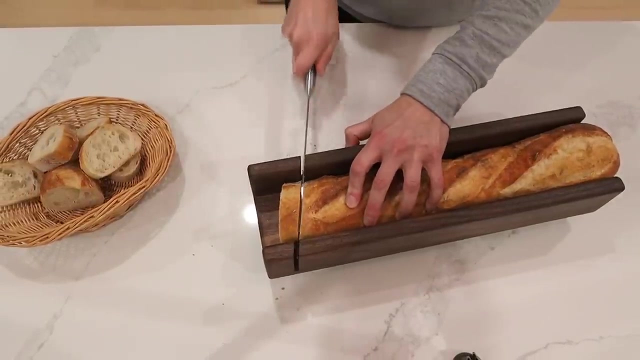 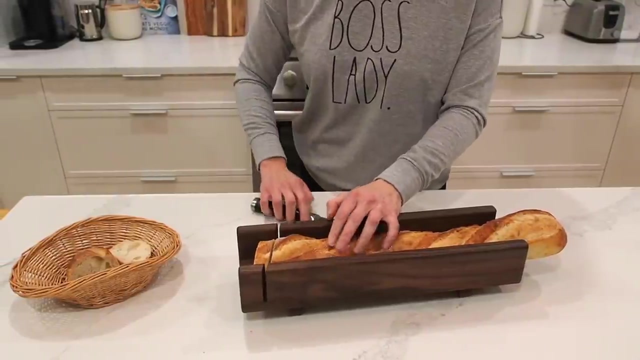 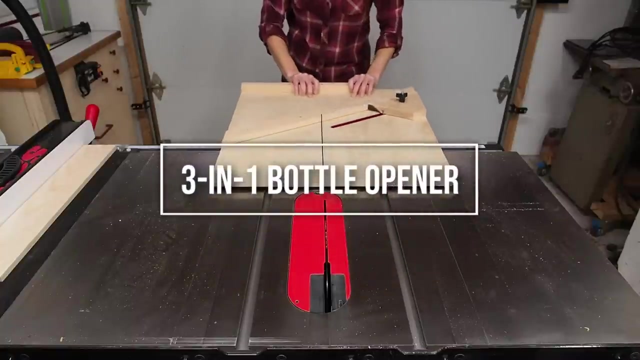 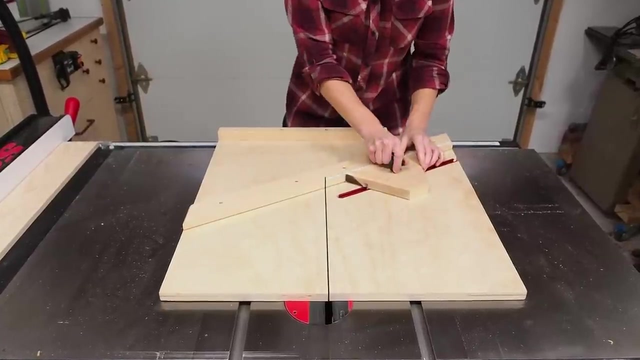 Now grab yourself a baguette and enjoy This one's a fun, easy project for all the beer lovers in your life. Now you can make this bottle opener any shape you want, but if you've watched any of my previous videos, you know I have a thing for hexagons. 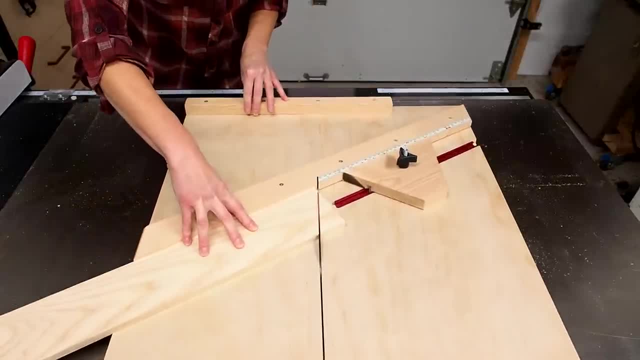 I built this hexagon jig using this old metal bar. I'm using a little bit more than half of my time and effort to make this work. The reason I'm using a bar is because I'm going to be making these for the first time in a while. 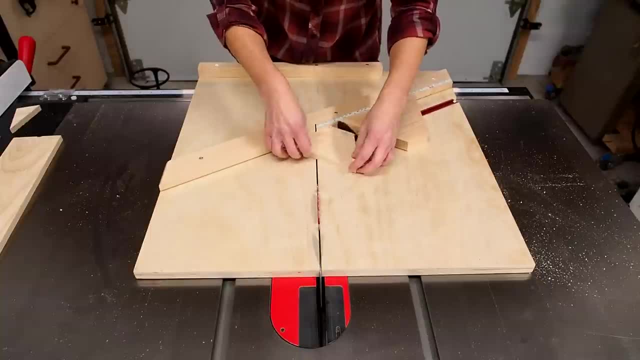 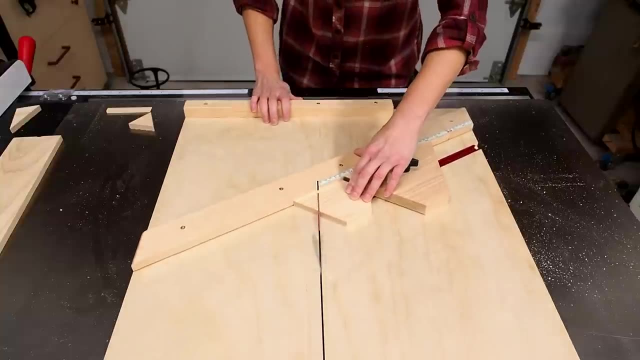 I built this hexagon jig a while back and I'll leave a link to it in the top right corner if you want to check it out. The cutting process is simple, Basically just cut, rotate and repeat. The idea is to insert this bottle opener right in the middle. so I'll start by connecting. 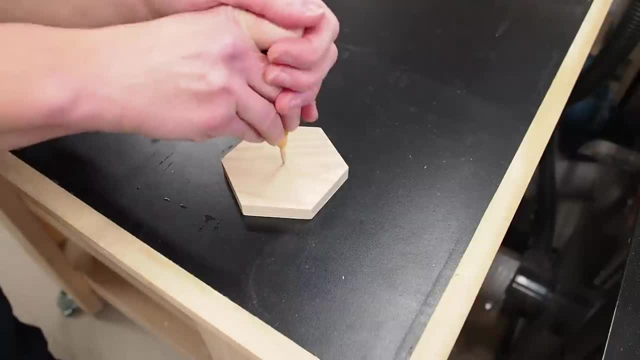 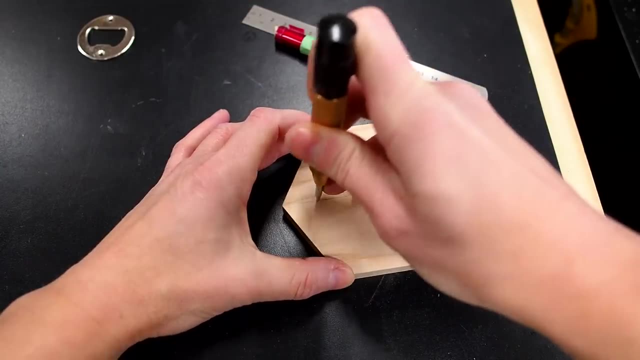 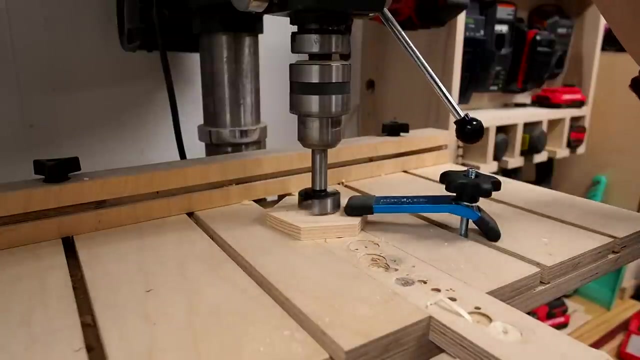 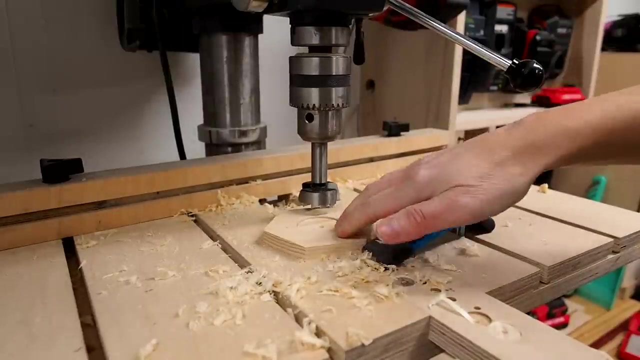 the opposite corners to find the exact center. Next I'll mark the spot for two magnets Alright over at the drill press. I'll start with a larger Forstner bit and make a very shallow hole. The closest bit size I have is 1-5-8, but you can invest in a 40mm bit if you plan to. 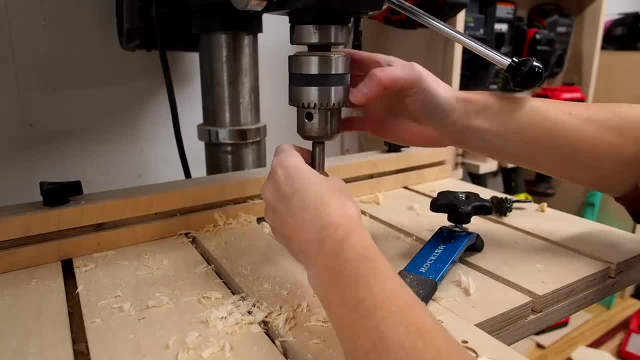 batch out a lot of these Looking good, so now I'll switch to a smaller bit and drill as deep as I can without poking through. It's a good idea to drill a little deeper than the first bit, so I'll just drill a little. 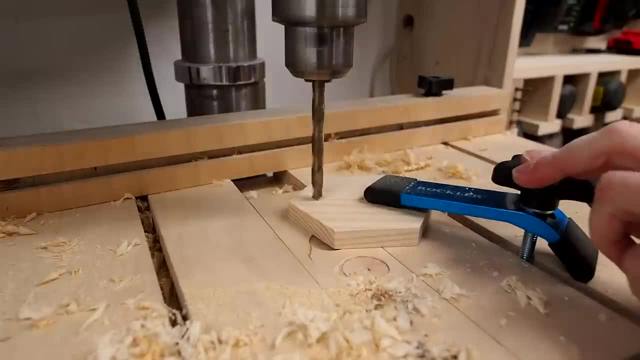 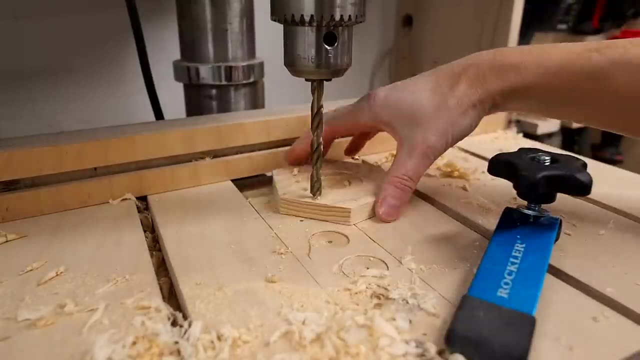 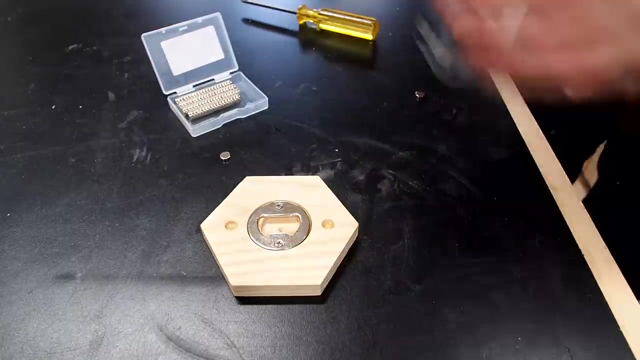 deeper. It's a good idea to practice on some scraps, first to dial in the settings And lastly, I'll drill the holes for the magnets. I'm using 8x3mm rare earth magnets that I got at Princess Auto To secure them. I'll apply a dab of CA glue in the holes and use the accelerator to lock. 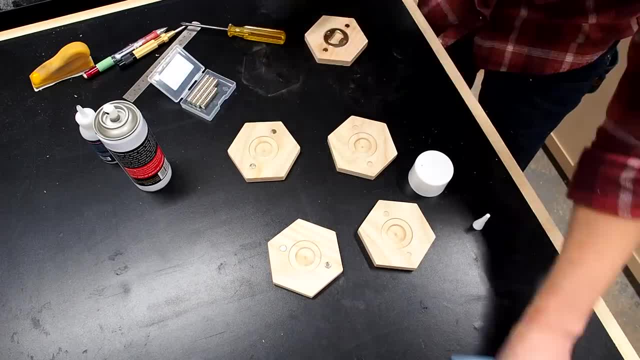 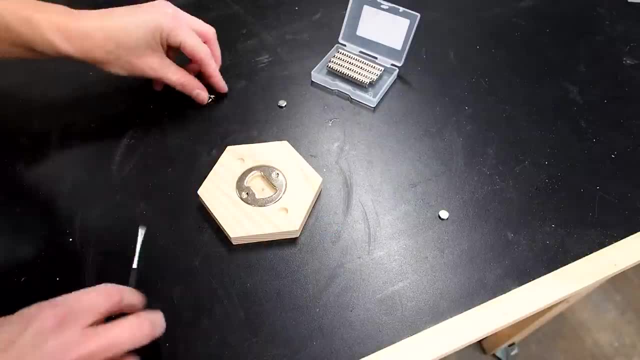 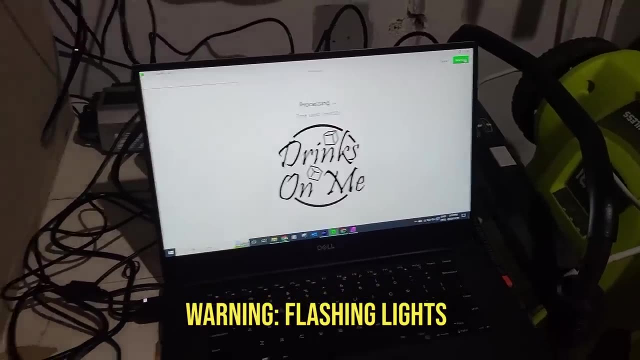 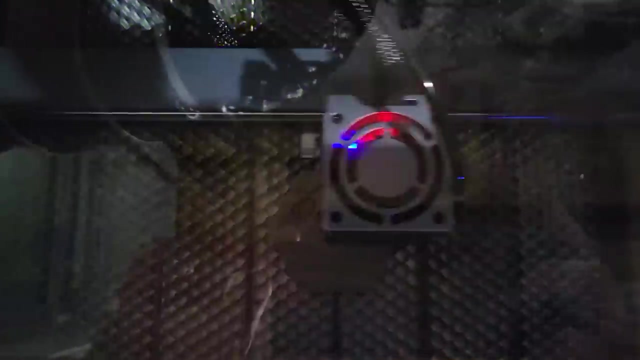 them in. I'll use a little more CA glue, then drop in the insert and secure it with the provided screws. Now you could stop here, but I got myself an early Christmas present that I couldn't resist trying out, So I designed this little logo and used my new laser to engrave the bottle opener. 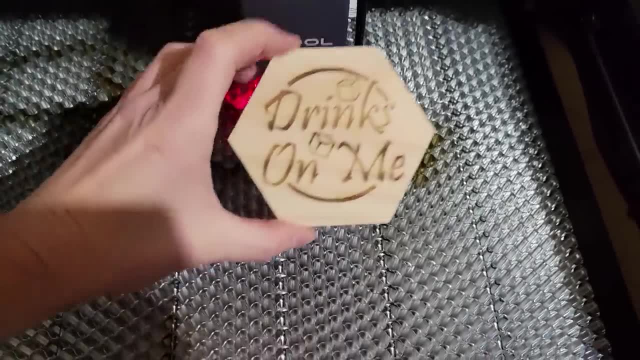 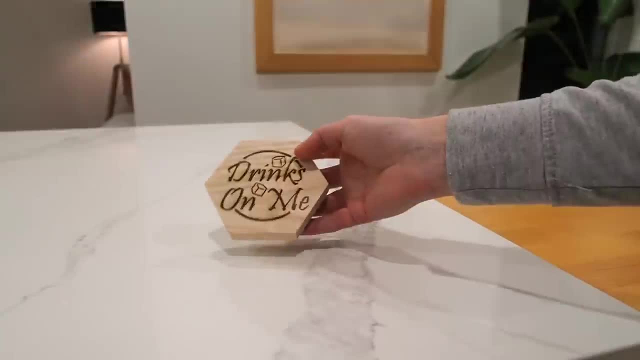 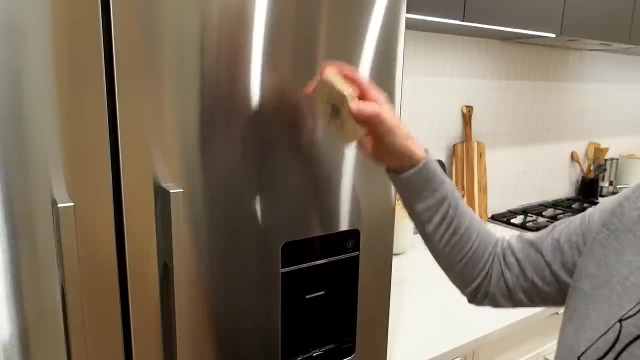 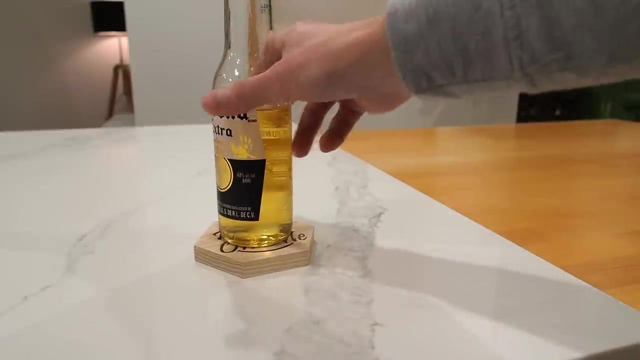 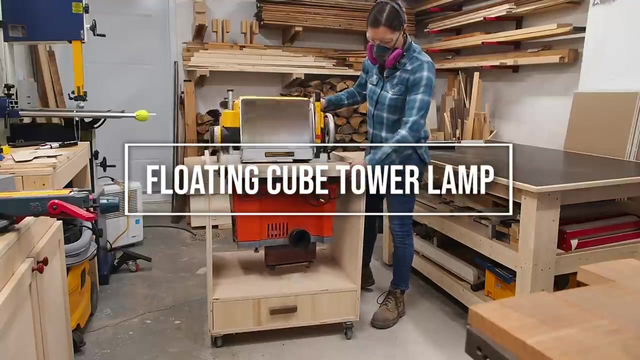 I think it came out pretty nice. Now all that's left is to pop open a cold one and enjoy. It's a bottle opener, it's a fridge magnet and a coaster all in one, And I love it. The next gift idea was inspired by a design I saw online that looked like a tower of floating. 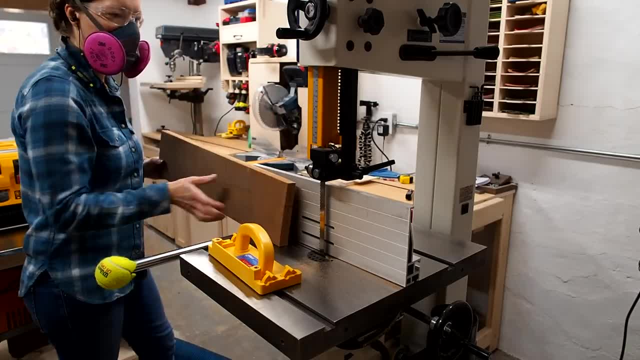 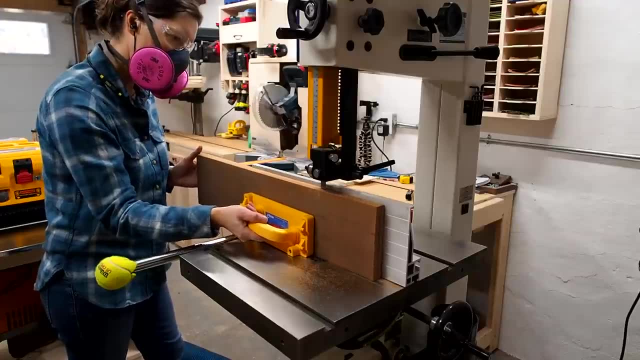 cubes with the light beaming up the tower from the base. There was no way I was going to keep this design I made. I just wanted it as a gift this year is pretty simple: Just make four open cubes and pile them up. I don't want it to be too chunky. 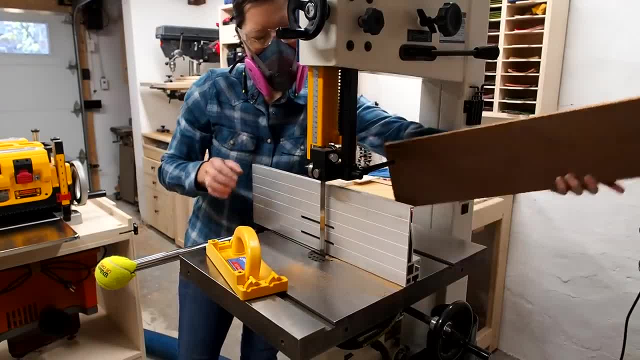 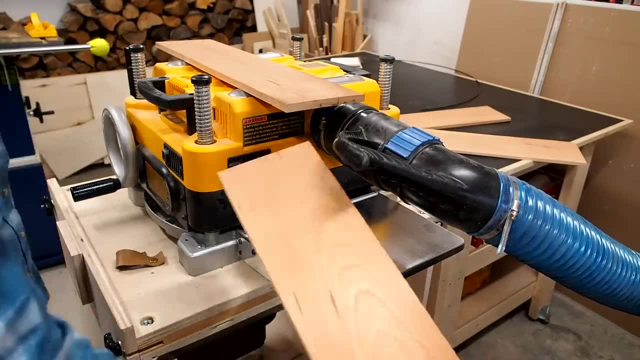 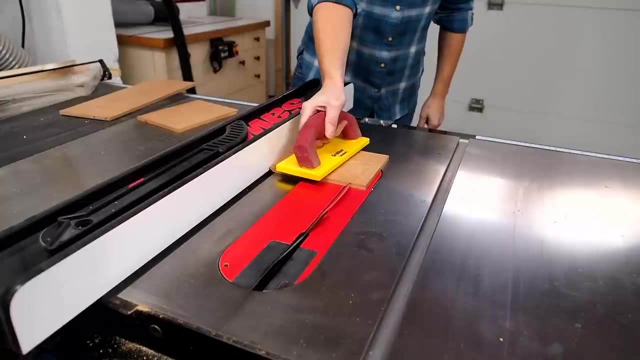 so I'm resawing some cherry wood into thinner pieces, which I'll then clean up on the planer. I'm going to create miter joints to assemble the boxes. so I'll start by tilting my blade to 45 degrees. Now you can simply run the pieces through like this, but it's not the safest or the 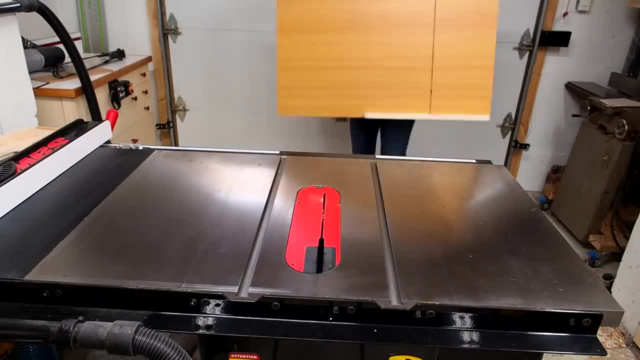 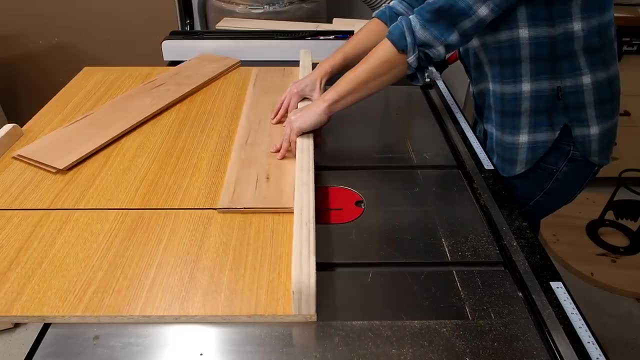 most accurate way to get a clean cut. So instead I'm going to use my 45 degree crosscut sled. It's basically a regular crosscut sled, but dedicated to cutting long miters or bevels. I'll first trim one edge off all my boards to create a reference edge. I can then set up a. 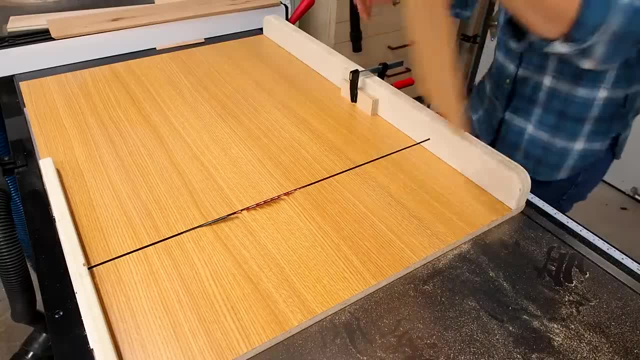 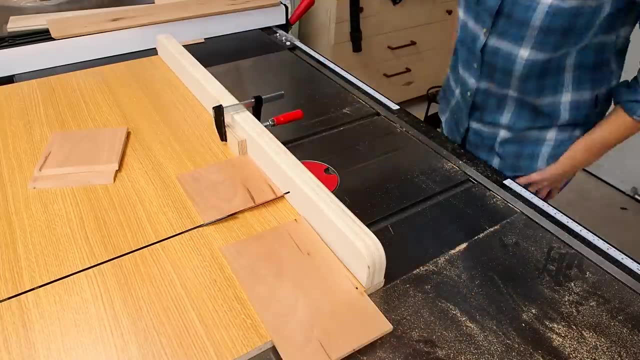 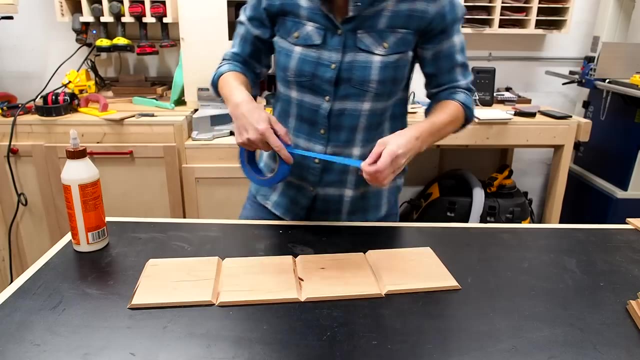 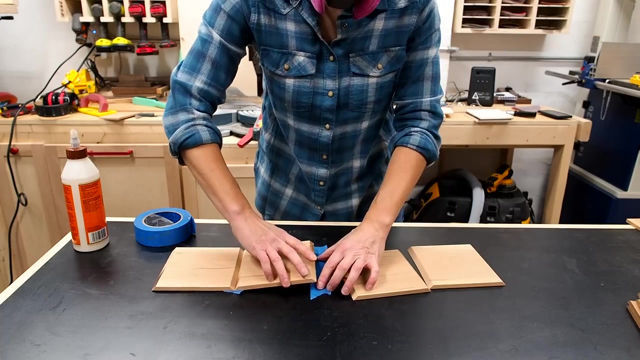 stop block so I can cut every single piece to the same length and end up with 16 identical pieces. Okay so, with all my pieces cut, it's time to assemble the cubes. The easiest way I've found to do this is to lay it all flat edge to edge. 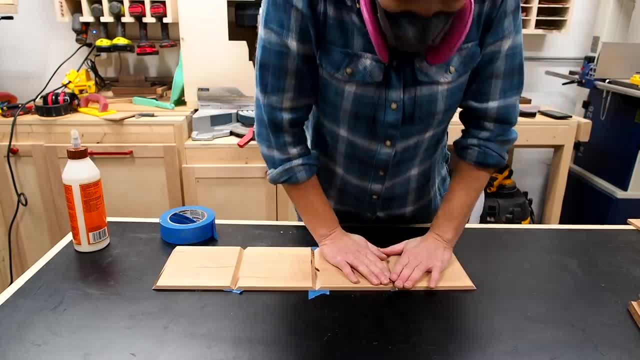 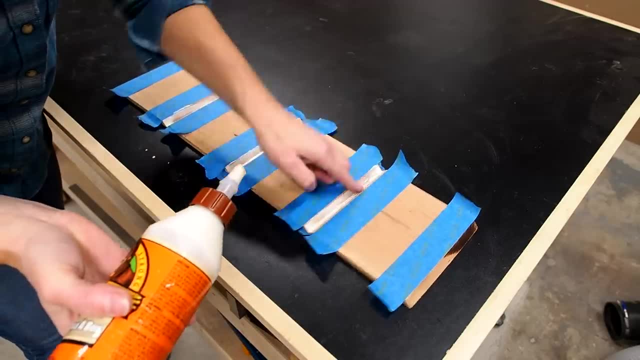 using some painter's tape to connect the edges. I'll then apply glue to the joints and fold it up into a cube. You'll notice a lot more tape here, and this is just to avoid having to clean up the squeeze out from the inside corners. Totally optional, but it definitely. 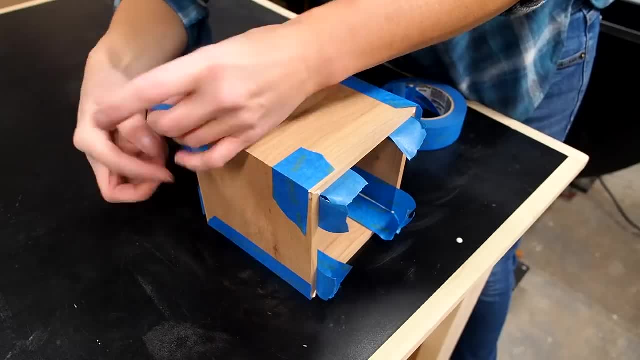 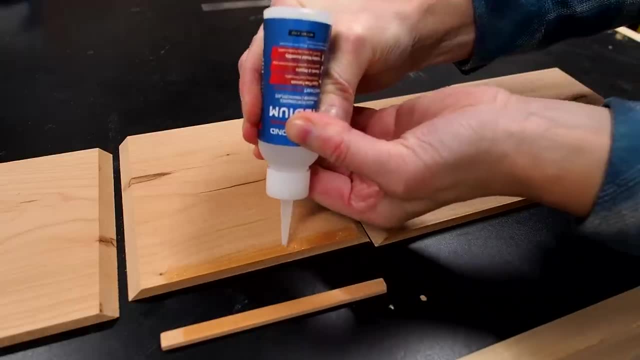 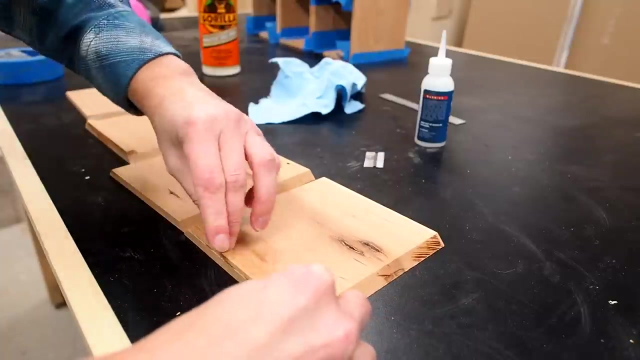 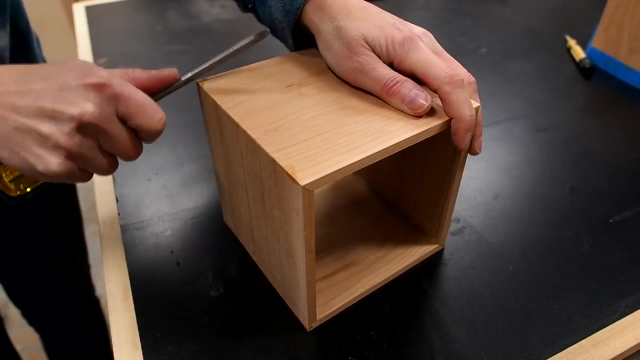 helps keep things clean. The bottom cube gets a small lip that'll support a floating bottom panel, and you'll see what that's all about in just a minute. Once dry, if you find that your miters are open, just use a screwdriver to press the edges together and close the gap. 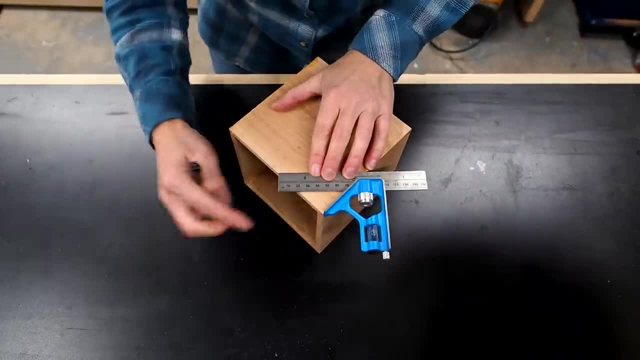 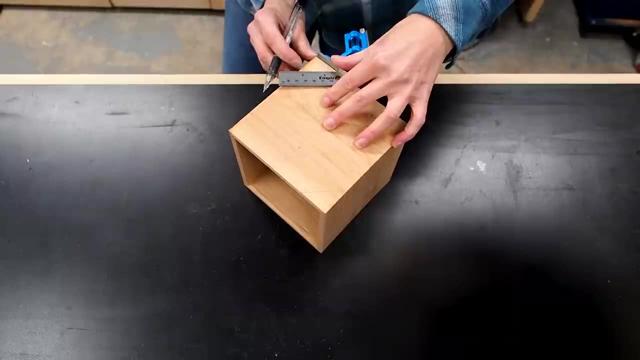 Okay, now we're getting to the tower part. Here I'm marking where the cubes need to be cut Now. this'll all make sense in a minute, but for now I'm just using the edge of my combination square as an arbitrary measurement. 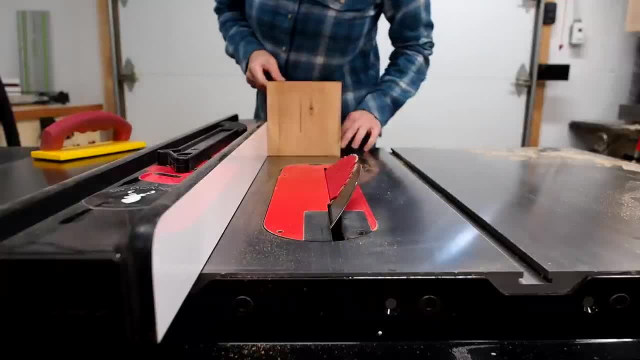 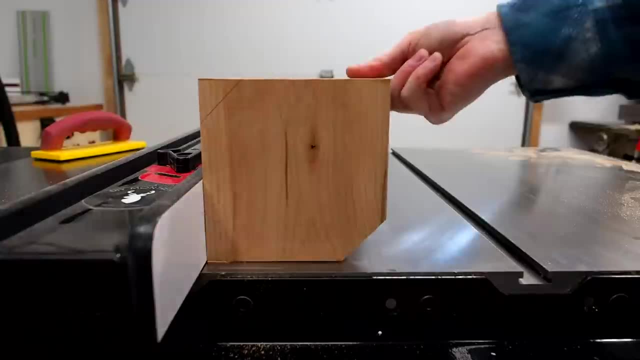 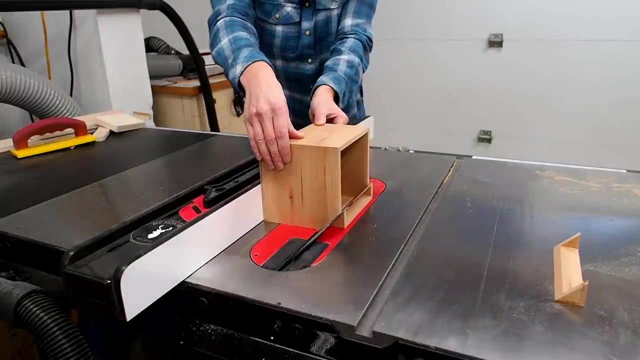 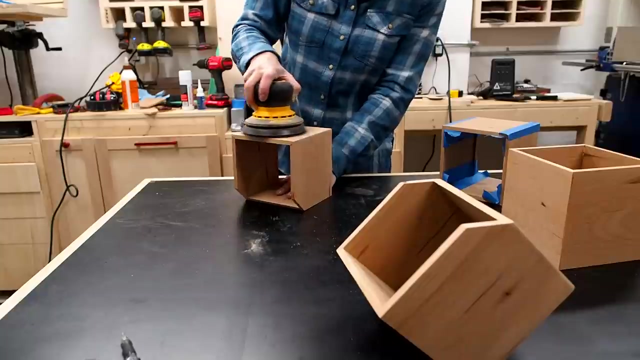 to make the mark. With my blade still set at 45,, I'll gently run the cube through and make the cut. For some reason this was super stressful, but it all turned out perfectly. Once assembled, it'll be really hard to sand this thing, so I'll just get that done while I still can. 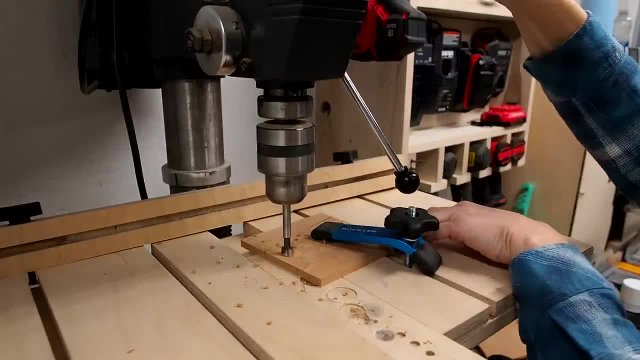 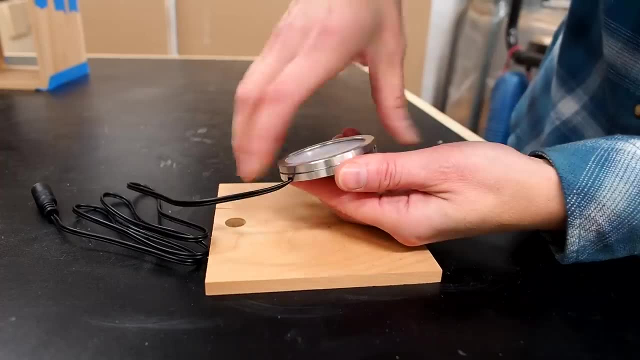 Okay, time to add the light source. I cut a panel to fit the bottom cube and here I'm making a small hole for the wiring. I'll be using an LED puck light that's probably meant to be used as cabinet lighting, but it'll work. It has a toggle switch, which will be perfect for a lamp. 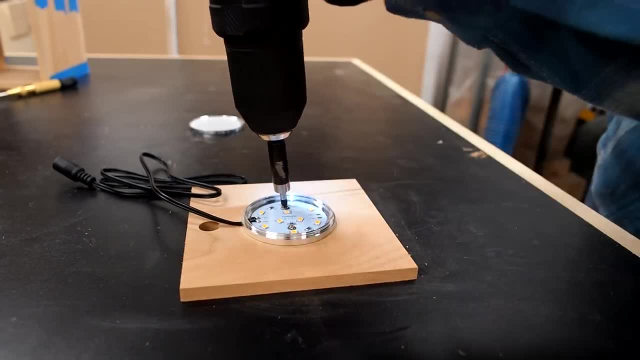 I'll just stick it on the top of the cube and then I'll make a small hole for the wiring. I'll just stick it on the top of the cube and then I'll make a small hole for the wiring. Secure it on center with the provided screws. 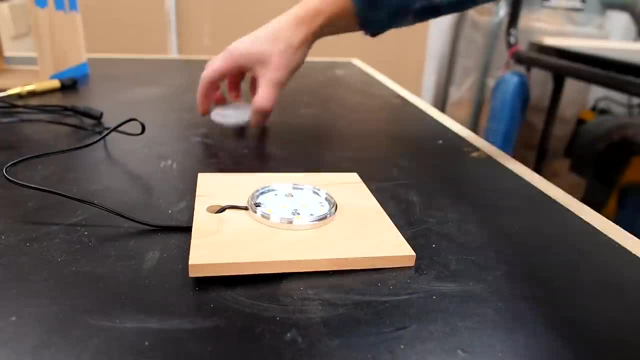 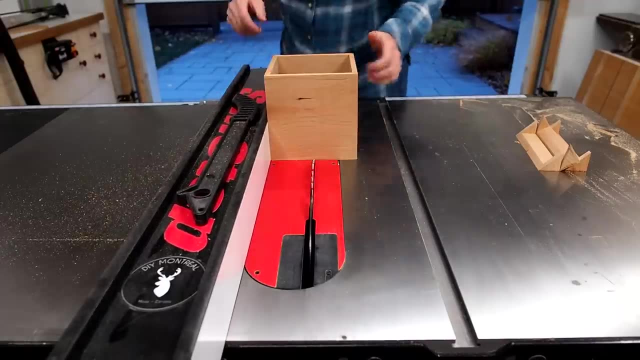 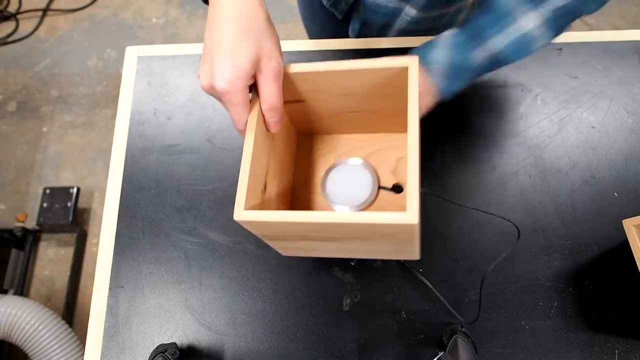 and thread the wire through the hole, Then seal it back up. One last thing is to make a small notch for the wire in the bottom cube by just running it through the table saw. Now I can drop in the panel and assemble this lamp. 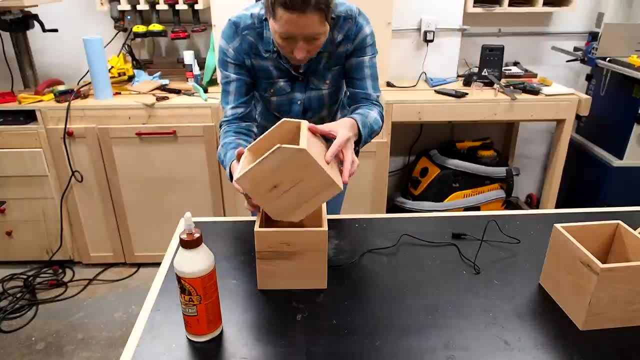 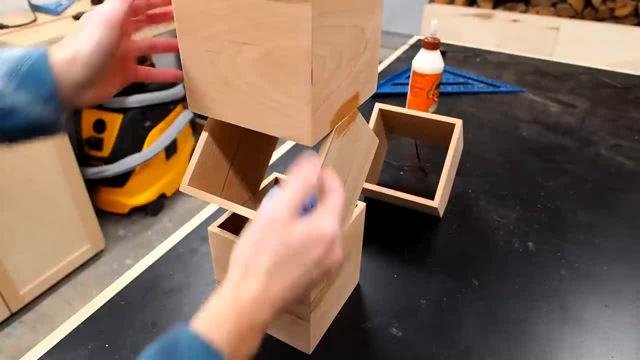 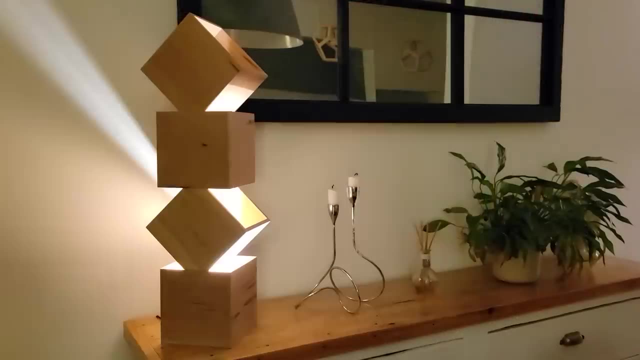 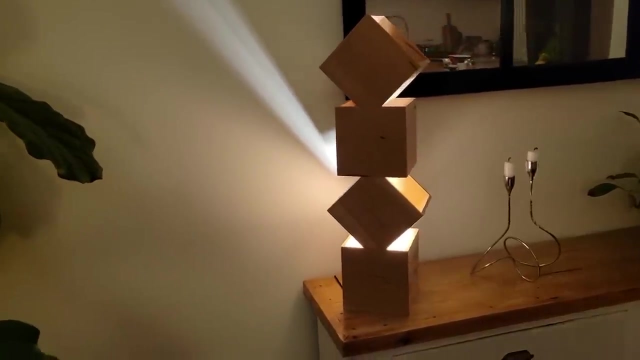 Just a few dabs of glue and a careful balancing act to build up the tower. I'm leaving it raw, but you can easily remove the bottom panel and apply a spray finish if you want. Okay, let's light her up PANTS. 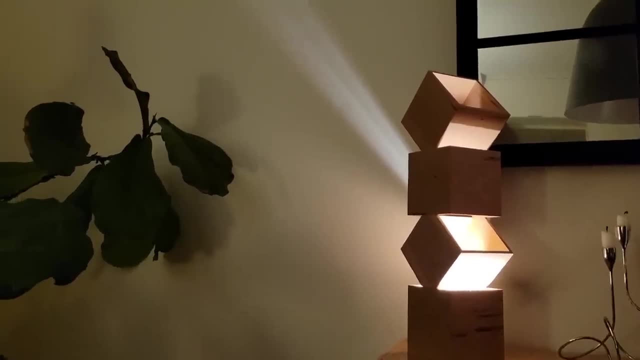 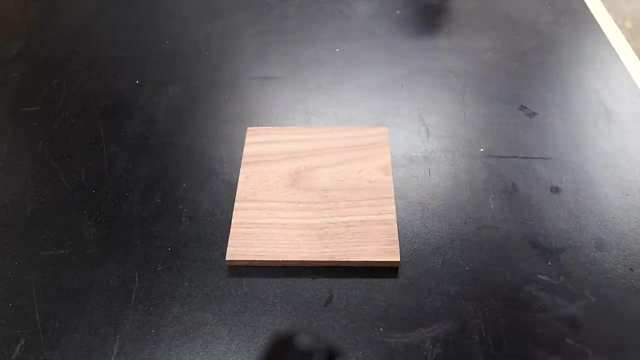 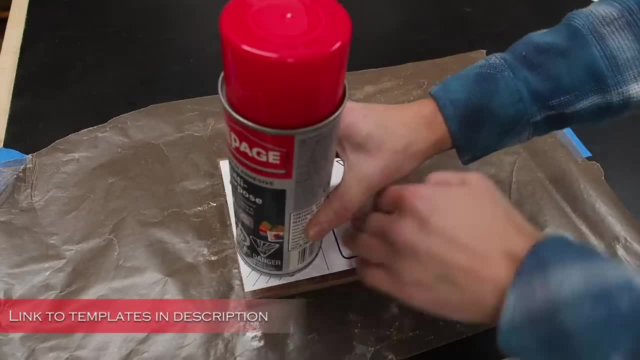 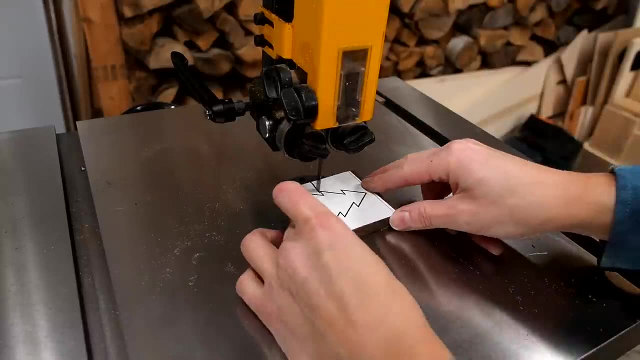 printed out. You can grab these for free on my website. I'll use some light spray adhesive to hold down the template so I can then cut out the shapes on the bandsaw. If you don't have a bandsaw, this might be difficult. The shapes are. 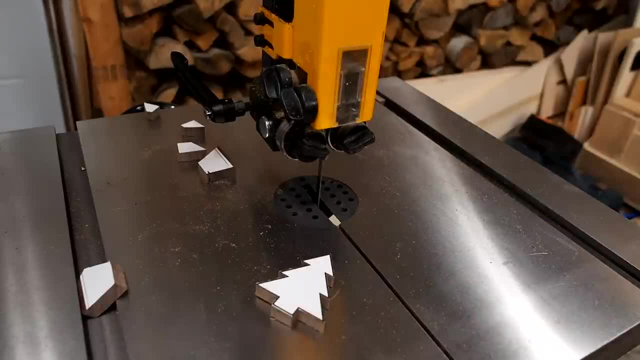 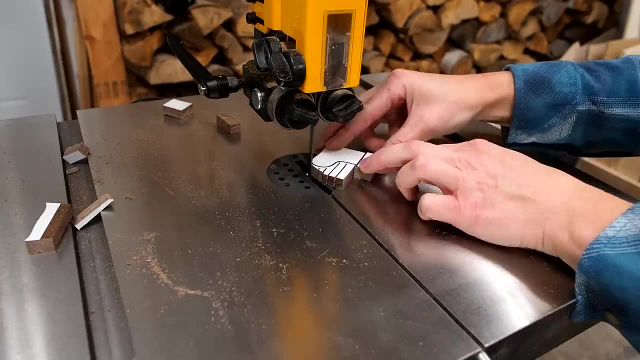 too small for a jigsaw, but if you have access to a laser cutter or a CNC, then you can cut these out cleanly. As for me, I'll do the best that I can on the bandsaw using a thin quarter-inch blade. Cutting the curves is a little harder. 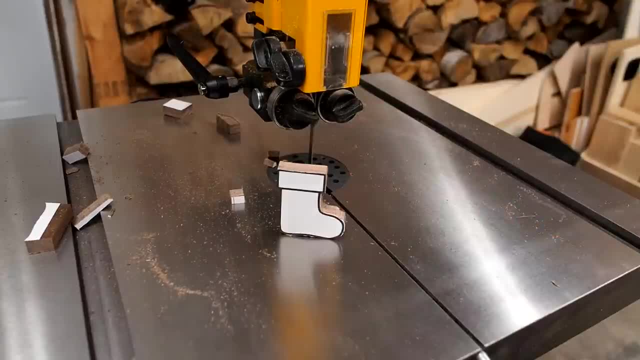 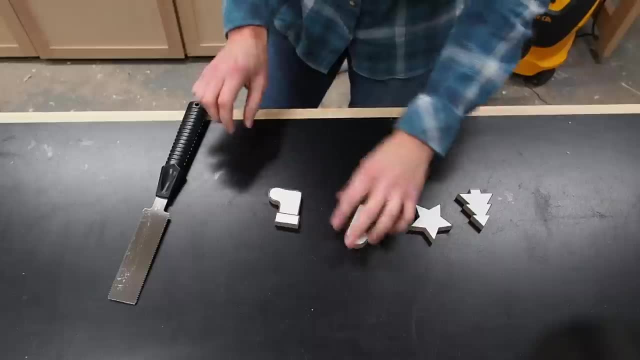 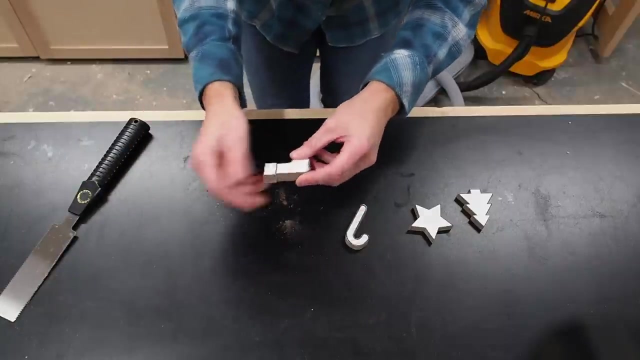 but I seem to be getting better at this. Maybe, Since the bandsaw leaves ridges along the edges, I'll do a little sanding to clean up the shapes. You'll notice lines on the templates on top of the shapes, So the idea was to use a small saw to cut on the lines and create a bit of a 3D. 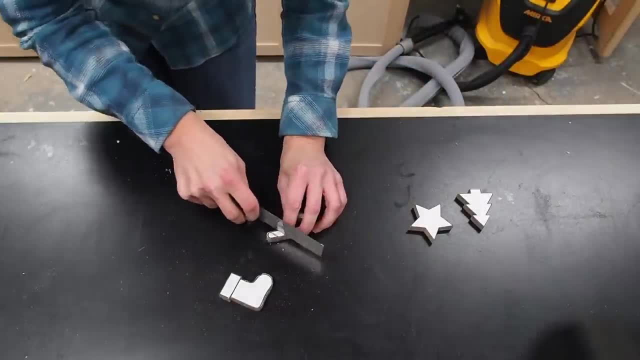 effect. I mean, you can't have a candy cane without stripes, right? You can't have a candy cane without stripes, right? You can't have a candy cane without stripes, right. We'll see how it turns out in the end, but I'm hopeful. 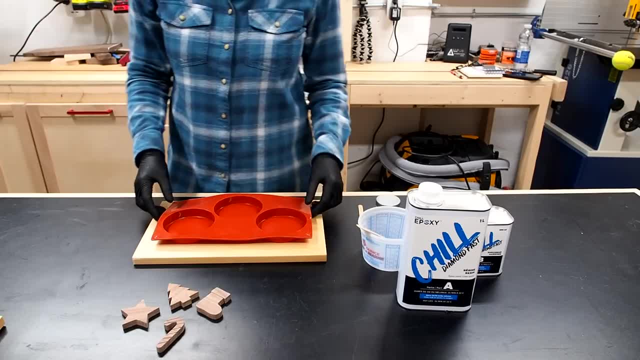 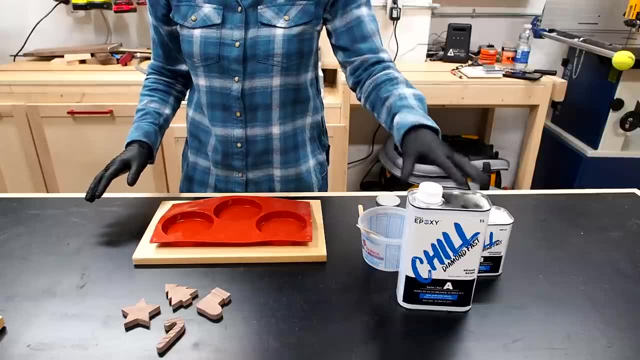 Alright, with that done, it's time to pour these coasters. I've got these silicone molds, my shapes and some fast curing epoxy, Oh and, of course, some white pigment for a winter snow effect. I'll leave links to all of these down in the 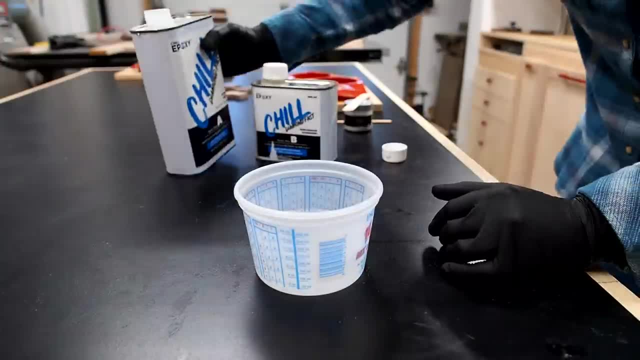 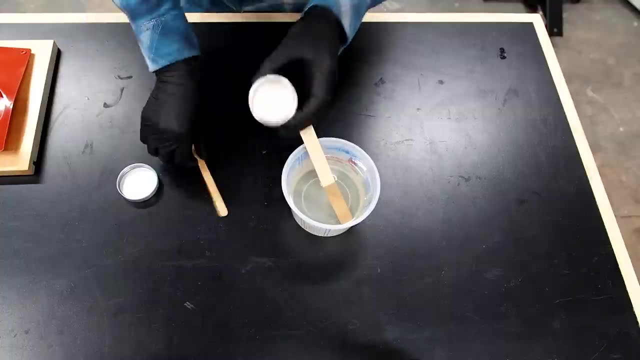 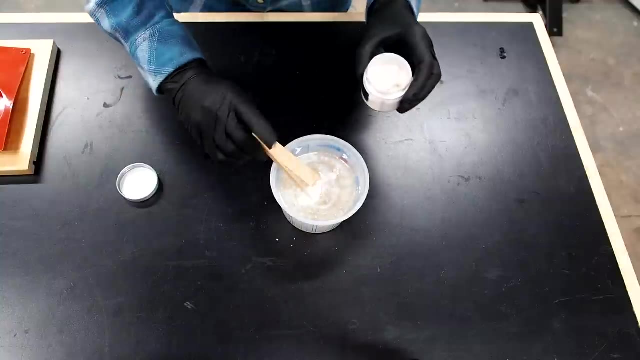 description below. Working with epoxy isn't as hard as you think. Just mix both parts in a cup, in this case two parts A and one part B- then mix it up. Then I can add my white metallic pigment and then maybe some more until I'm happy with the. 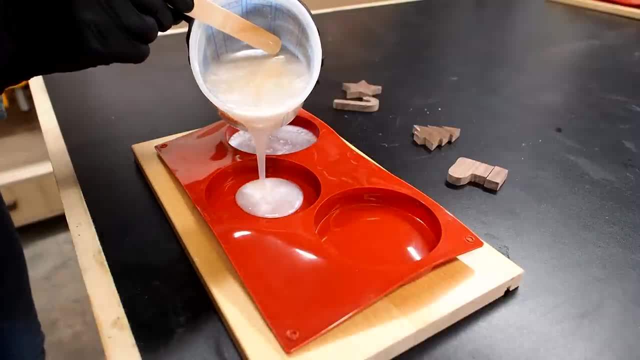 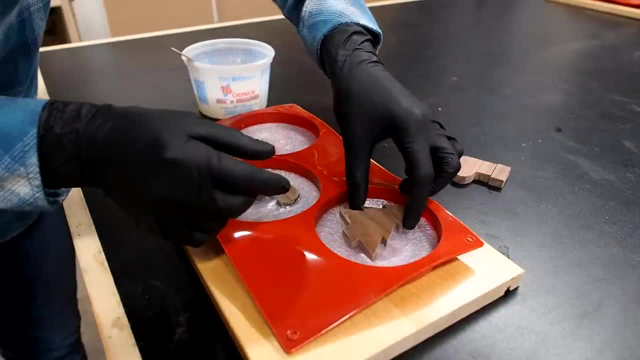 color. I'll first pour a thin base and then drop in the shapes face down and move them around a little to make sure no air pockets get trapped in those lines I cut. I can then top them up, but no need to go all the way to the top of. 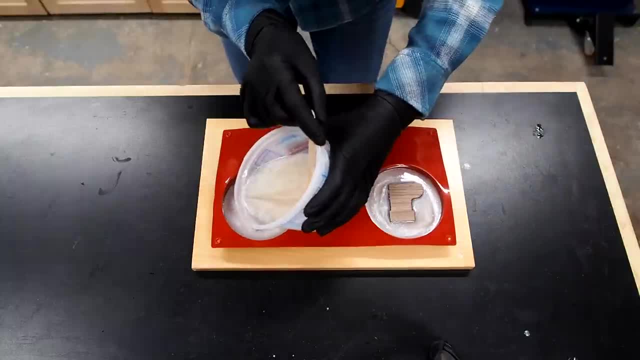 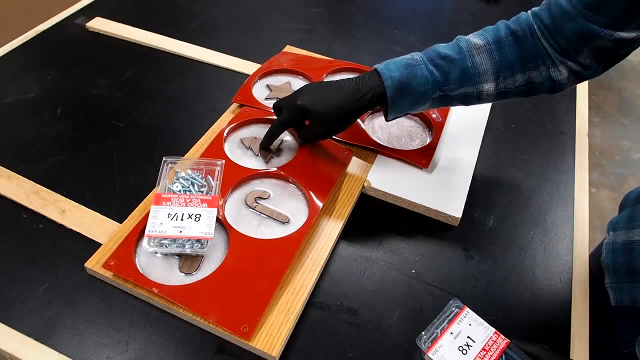 the shapes. We'll be sanding those down later. The wood will want to float around in the epoxy, So I found some weights that I'll use to hold them in place while the epoxy cures Anything. plastic is a good option for this. The next day I can easily pop them. 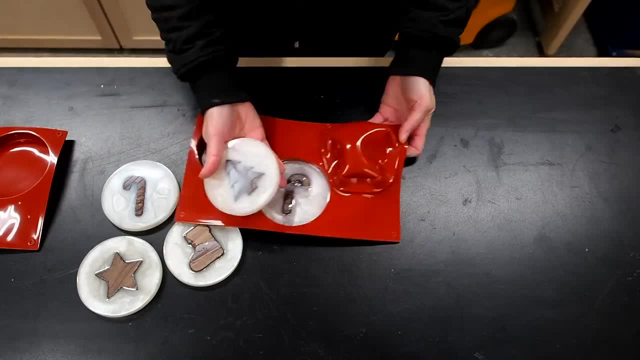 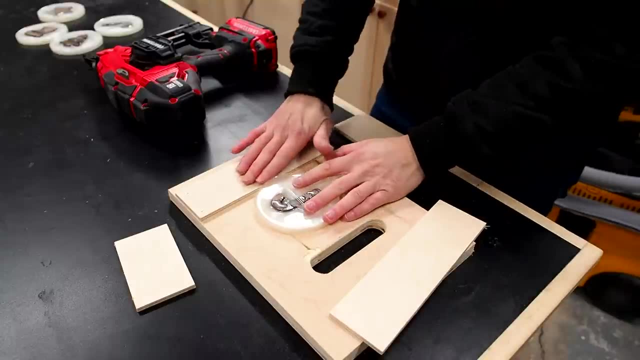 out. As you can see, they don't stick to the mold and they come out nice and easy. Now the idea is to get them all down to the same thickness, about a quarter inch. I'll use some scraps to make a simple sanding jig using quarter inch plywood. 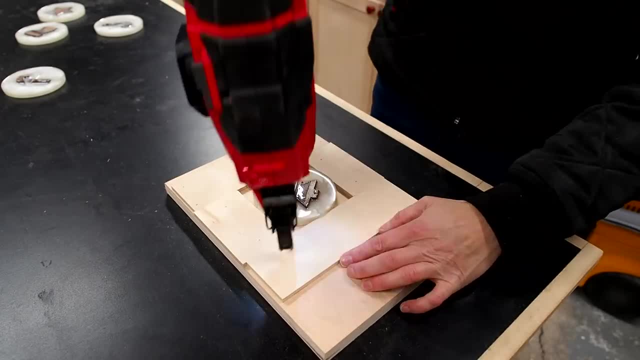 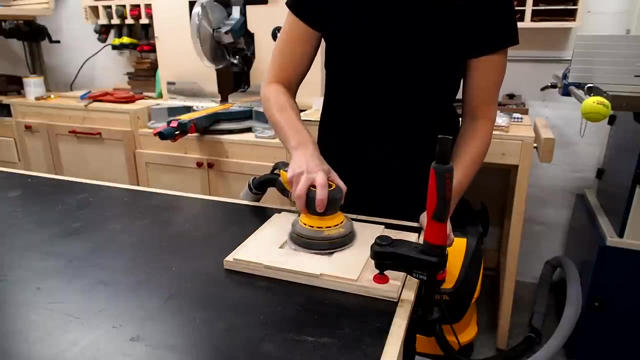 that'll surround the coasters and hold it in place while I sand them. This also happens to be the same thickness that I'm aiming for my coasters to be, which means I can just keep sanding, feeling the edges as I go, until. 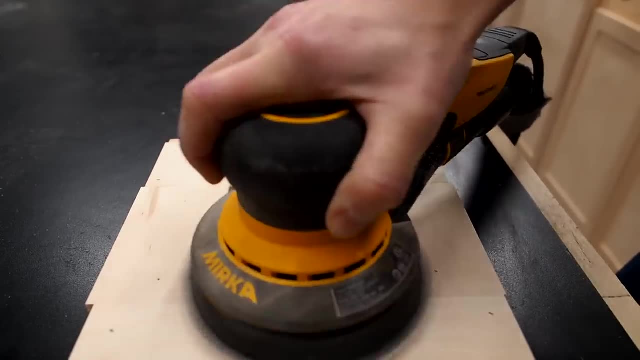 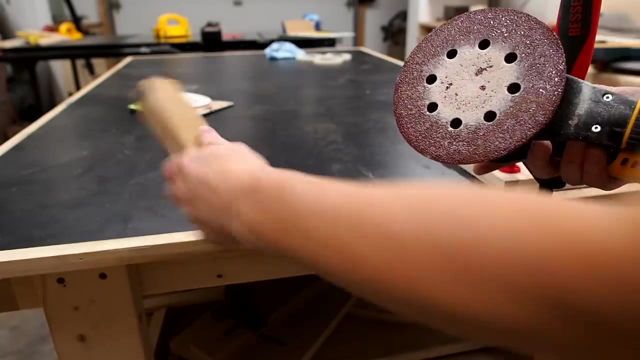 my sander bottoms out. I'm using 60 grit paper to really grind these down quickly. Just be careful that you don't overheat the resin or the shape might become a little deformed. It also helps to clean your sander, often using a. 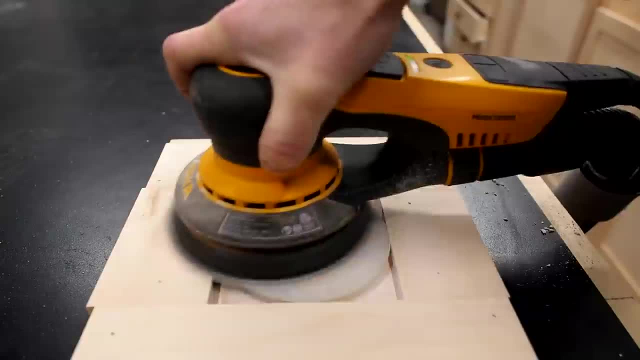 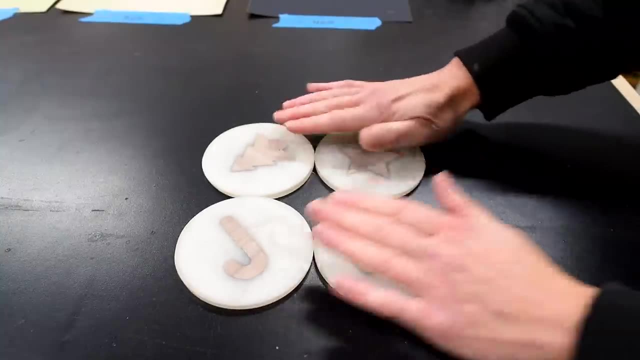 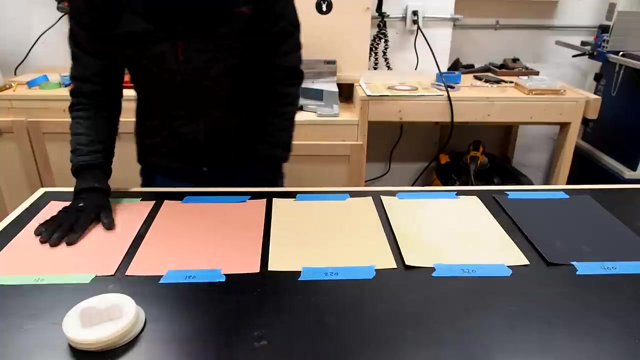 rubber cleaning block. Once all four are done, they should all be even in thickness. They're looking pretty rough though, so as a final touch I'll polish them up. I set up a series of grits from 120 to 180 to 220 to 320 and finally 400 grit. 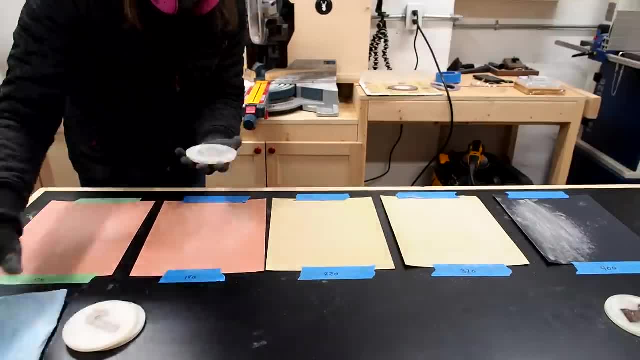 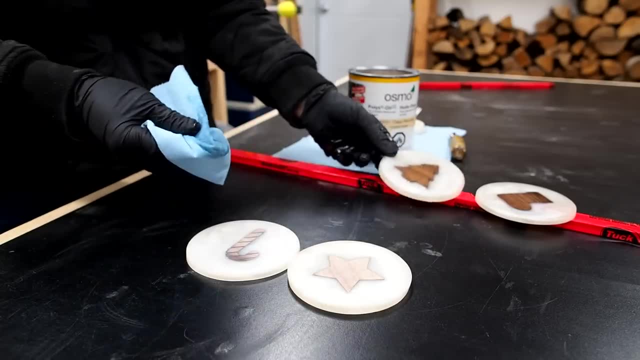 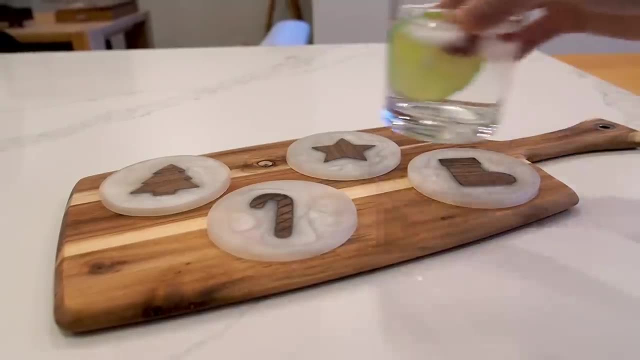 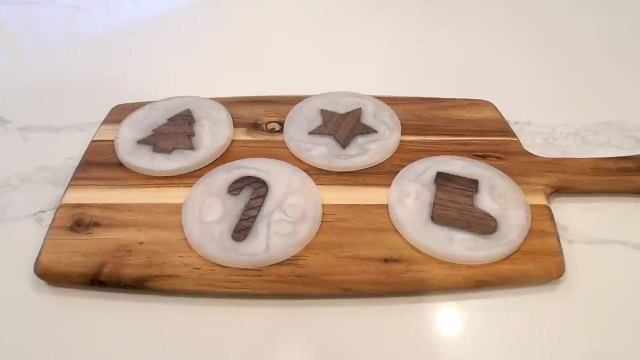 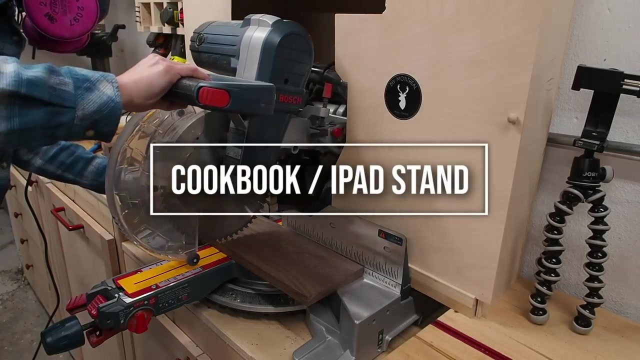 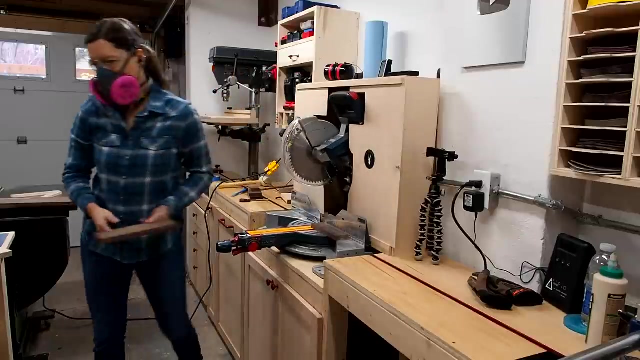 All that's left is to add some. finish, let it dry and enjoy. If anyone on your Christmas list loves to cook, this one's for you. I'm making a collapsible cookbook-slash-iPad stand that can also be used as a serving. 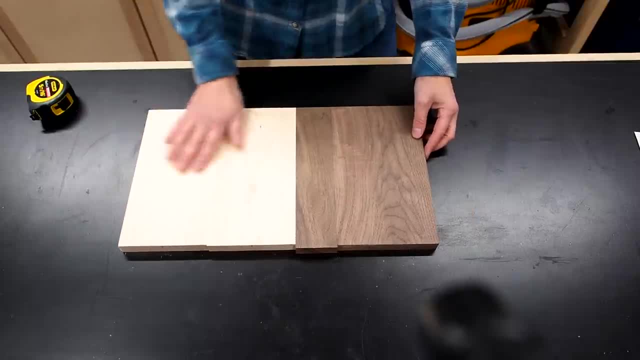 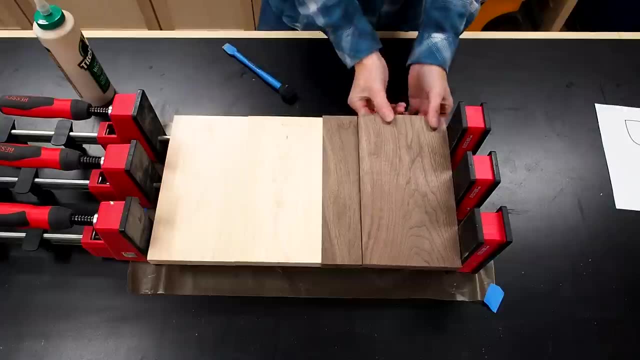 board. I cut up some walnut and some maple and found a layout that I liked. It should be roughly 16 inches long by 9 inches wide. give or take Again, all the dimensions will be available on my website, Just like making a cutting board. 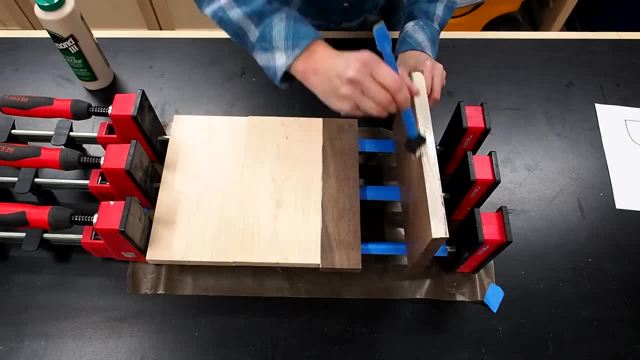 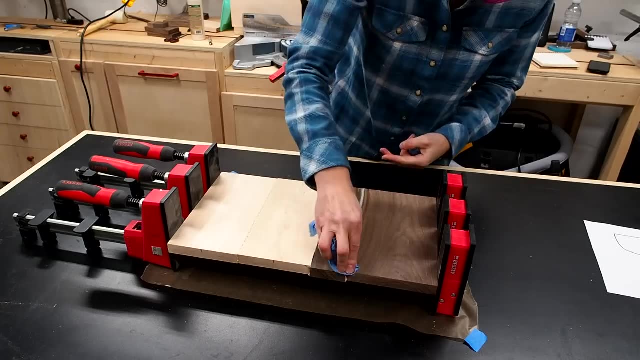 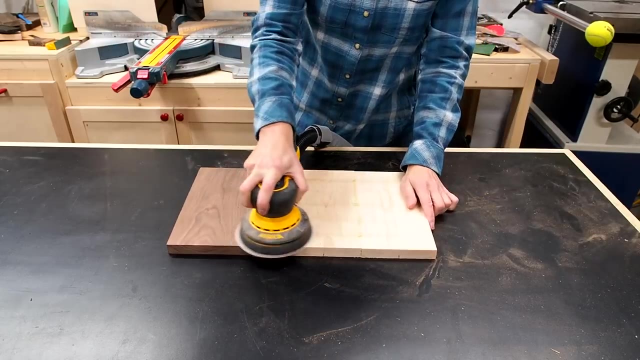 I'll apply a generous amount of glue to the seams and clamp them all together. I won't be using the planer for this, so I made sure to wipe away all the glue with a damp rag. Once dry, I sanded with 80 grit just to get the faces nice and flat. 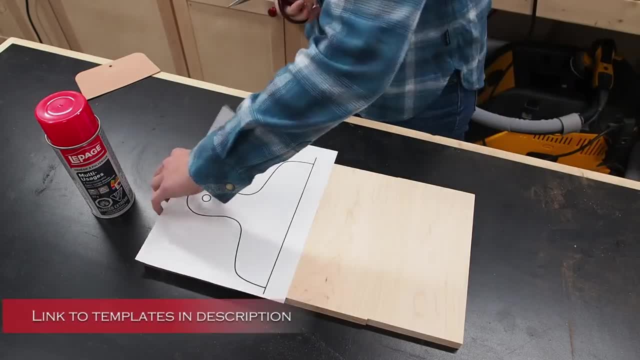 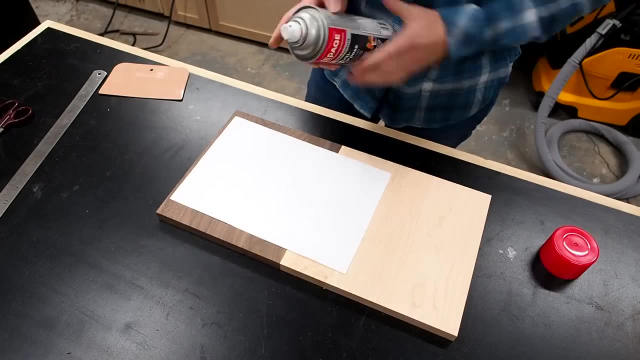 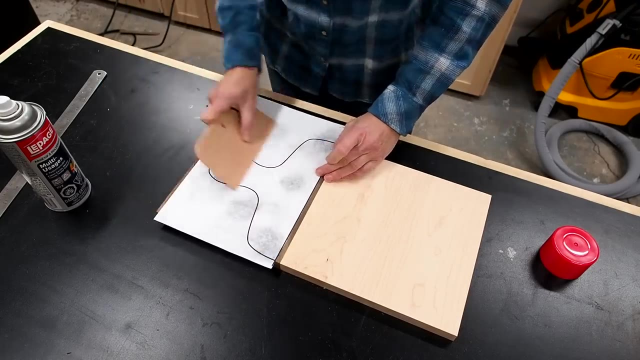 I designed this cutting board handle on the computer to make a printable template, and you can download it for free on my website. I'll leave a link down below. Using some light spray adhesive, I'll secure the template to the wood and press it down. 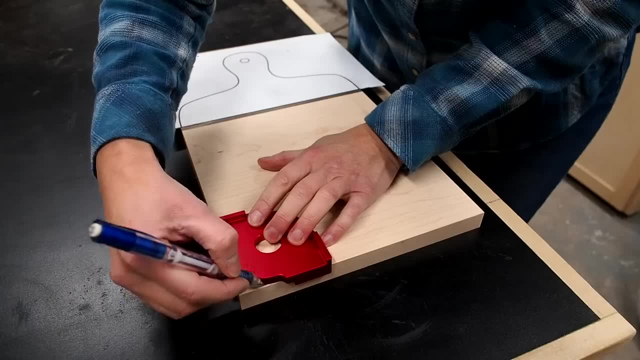 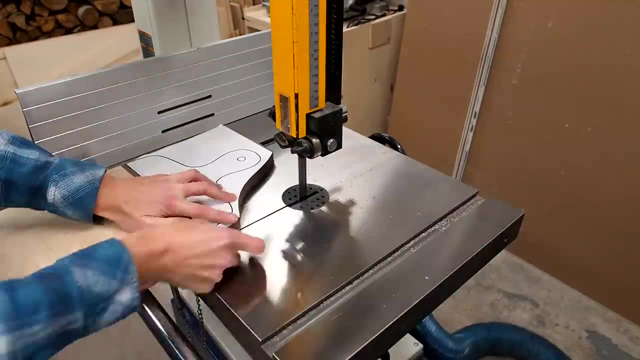 I'm using this radius jig to round the bottom corners, but I like to use it as a guide to. but you can use any circular object that you have on hand, like a bottle cap or whatever. I'll use my bandsaw to cut out the handle. Now I'm a little embarrassed to show you this, actually. 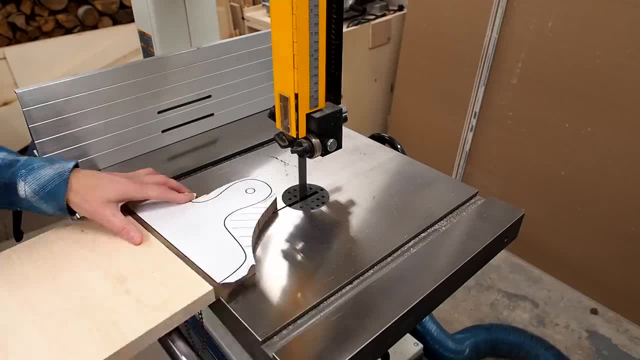 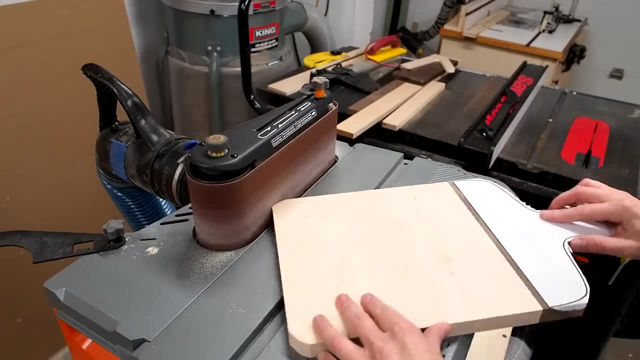 because, one, I was too lazy to change my blade and this resaw blade is making it impossible to cut curves, And two, I probably could have and should have just used the jigsaw to do this. It likely would have been a lot faster and a lot cleaner, But luckily for me, there's nothing a. 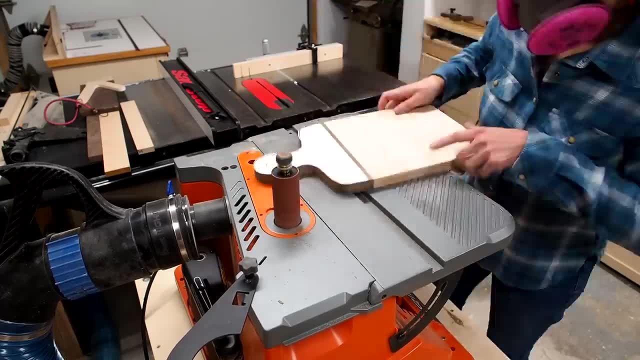 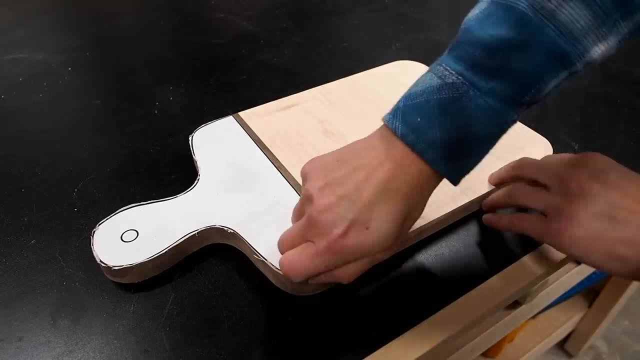 little sanding can't fix. I started by smoothing out the lower corners, then used the spindle attachment to refine the shape of the handle Much better. At this point I didn't even notice that I forgot to drill the hole in the handle before pulling off the template. 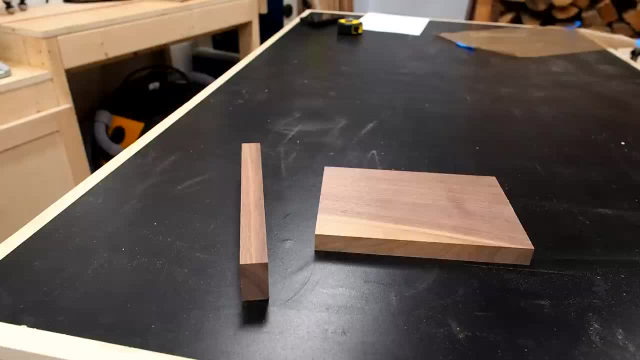 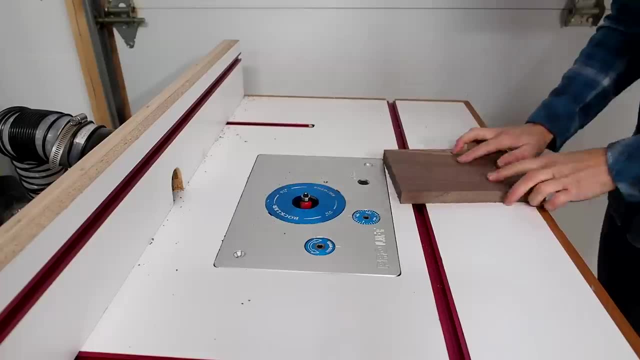 but I'll go back and do that later. Moving on to the other half of this stand, I'm going to attach these two pieces of walnut into a t-shape, But first I want to break all the sharp edges, so I'll round over all the edges on the router table. 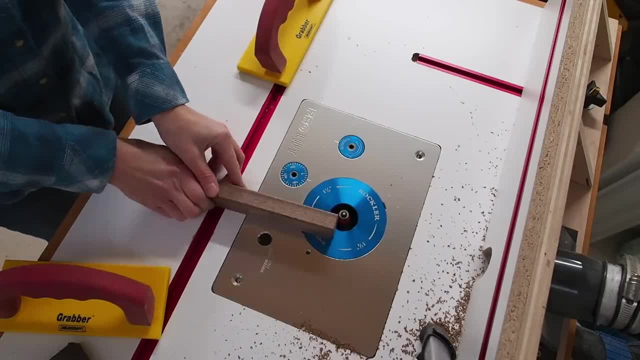 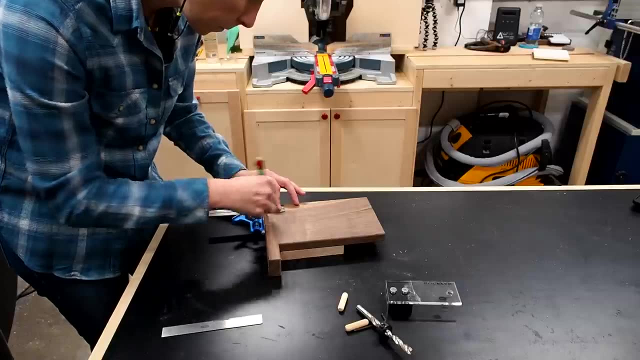 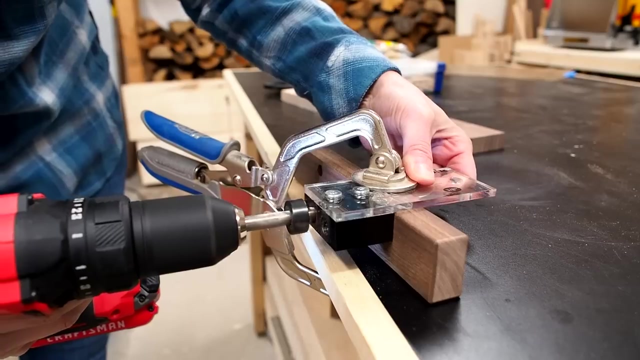 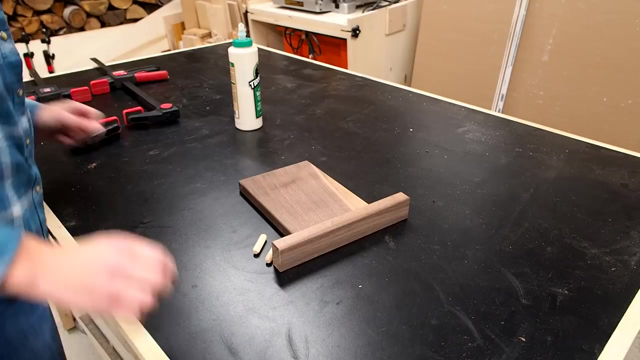 To assemble them. I'll use some dowels. Here I'm tracing some simple layout lines that I can use as a reference for my doweling jig. I'll add a little glue And, by the way, for kitchen items that might get washed, 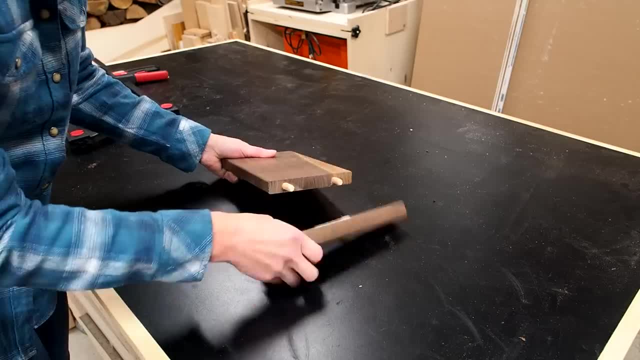 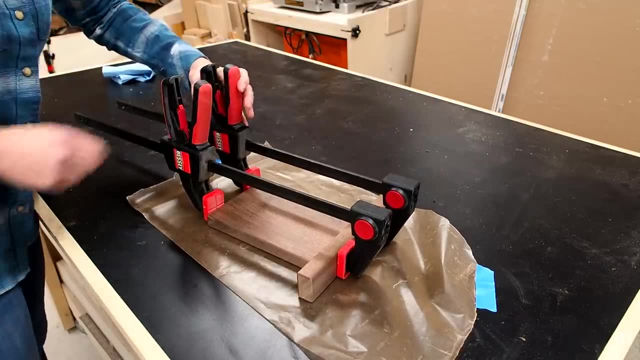 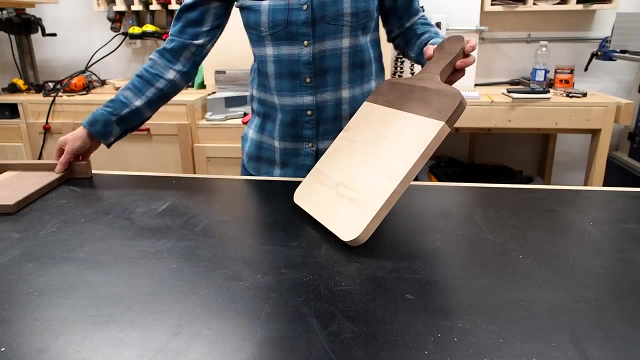 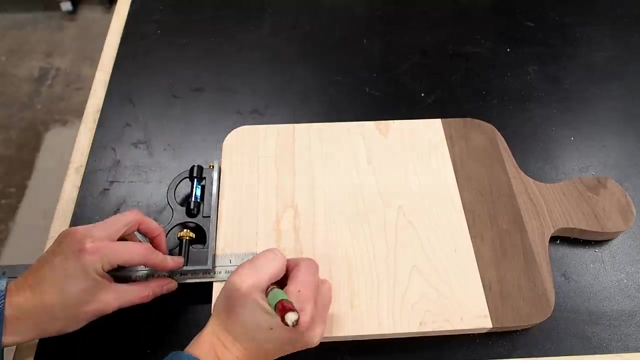 I always like to use a waterproof glue-like type bond 3.. I'll add some clamps and let that dry. The last step is to cut a slot in the board to fit the stand. First I'll roughly mark the width of the slot, then use those as a reference to trace out the slot. 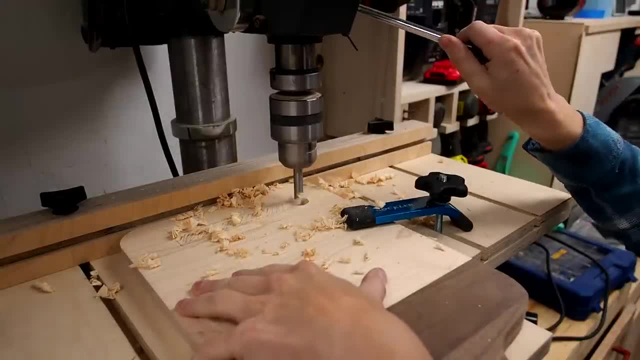 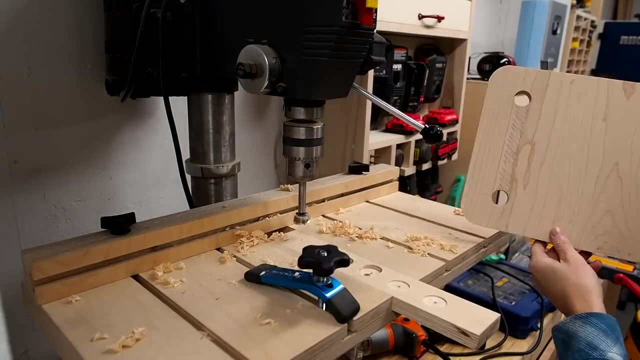 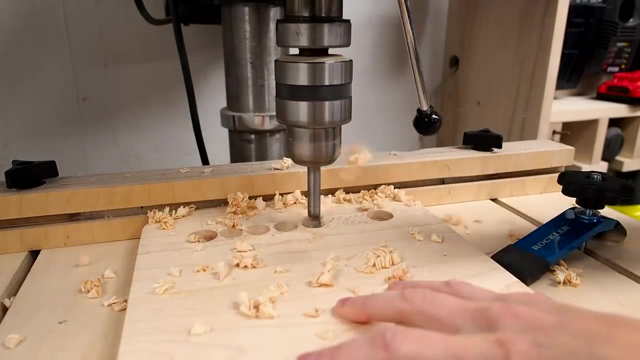 I'll use a forstner bit at each end and drill all the way through. Next I'll switch to a smaller bit and remove most of the waste while staying inside the line. I can now use a router with a guide and an up spiral bit to finish cutting the slot. 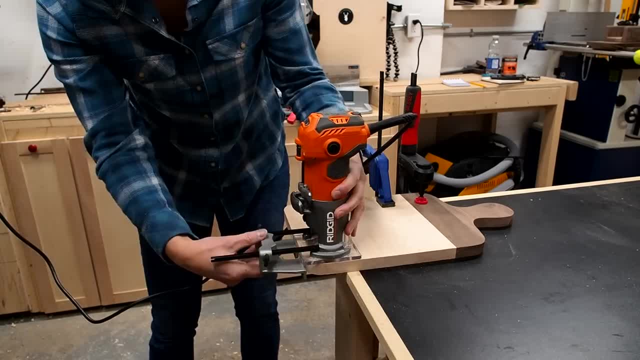 I'll push the bit up against one side, then lock down the guide rail. Now I can fire up the router and run it along the first side and then run it along the first side, and then run it along the first side and then run it along the first side. 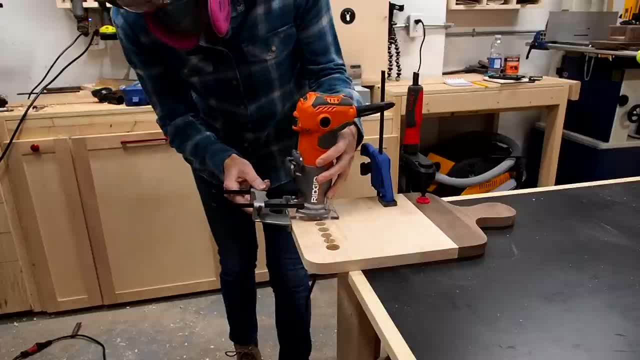 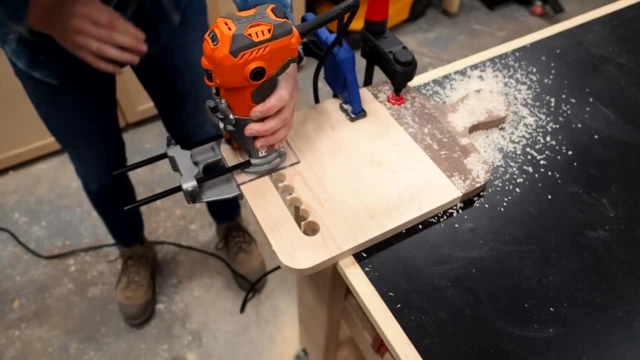 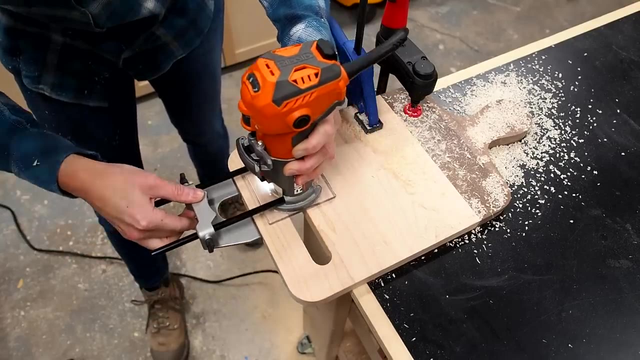 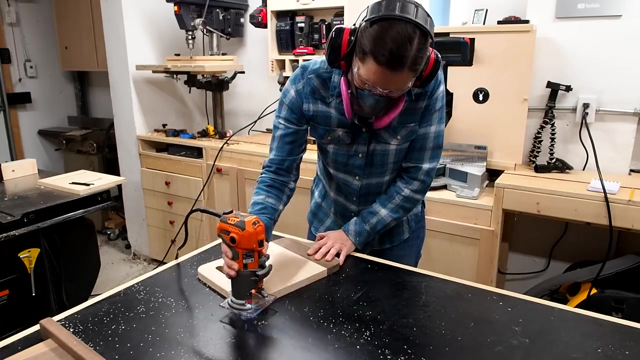 then progressively lower the bit and run it again until I'm all the way through, Then repeat the same process on the other side and voila- perfect slot. All that's left at this point are the finishing touches, like rounding over all the edges. 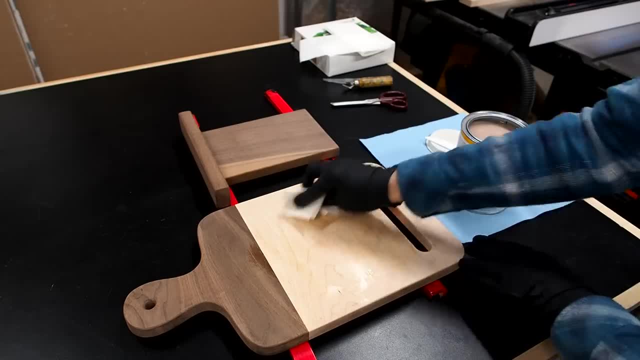 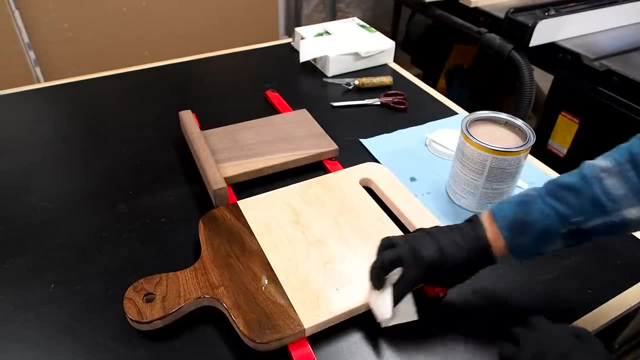 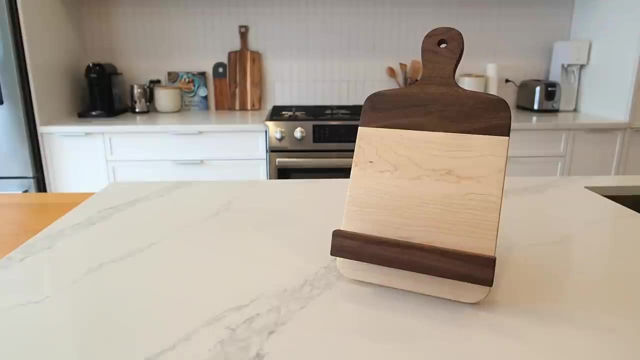 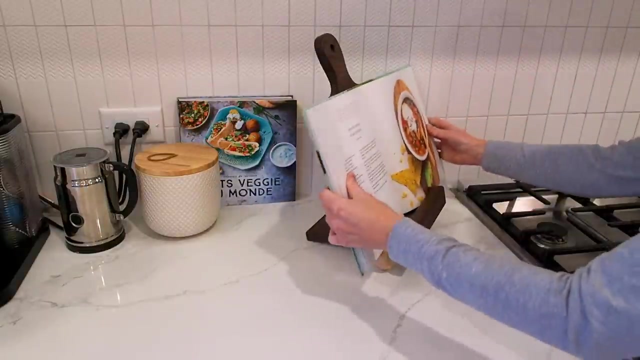 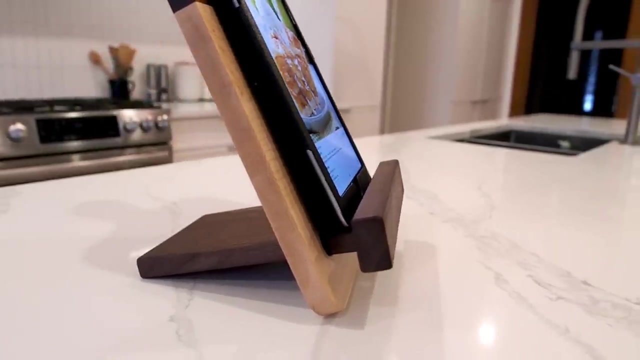 sanding and applying a finish. Again, I'm using Osmo Pollux oil just because it's a no-brainer wipe-on finish that's low VOC and can be done in a single day. Now find your favorite recipe and enjoy Ounk. 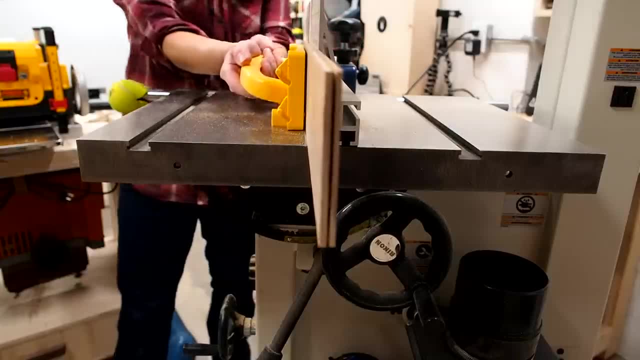 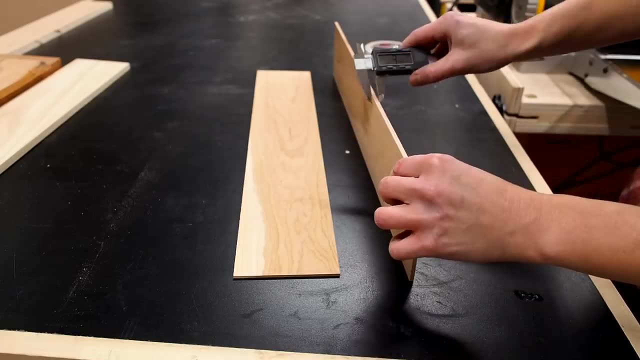 The next one is really simple, but if you wanna give a little hand, made something to a lot people in your life, this one might be right up your alley. Bookmarks, Yes, bookmarks. For this you'll want really thin wood like. 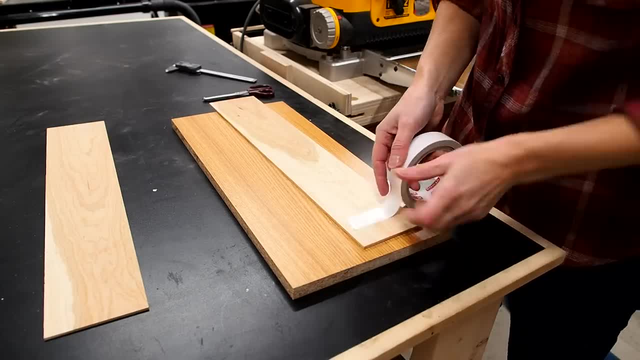 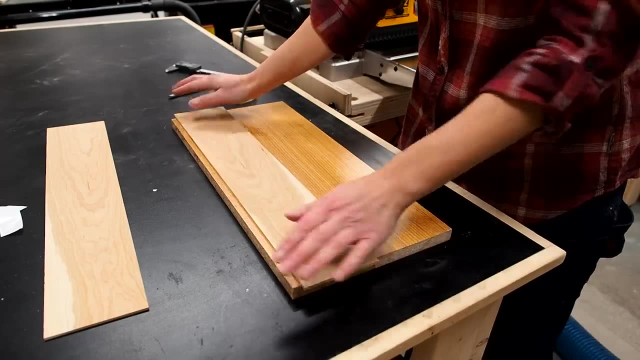 but I wanted to try using solid wood. The bandsaw leaves rough marks and my pieces aren't even in thickness. But I can't run these pieces through the planer, they're just too thin. A simple trick is to use a piece of particle board and stick down the pieces with some double-sided